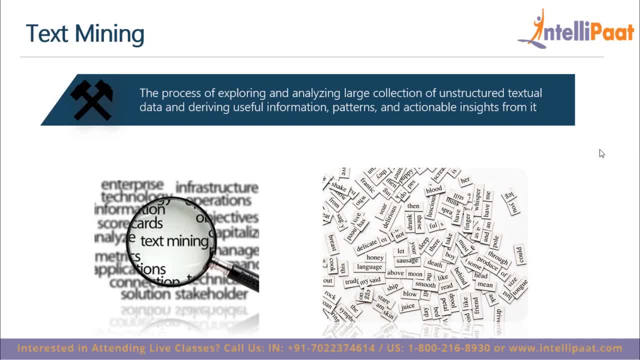 which ends with the number 30. Now you have absolutely no idea what that number means. It could be the number of days in a month, the amount of dollars a stock increased over the past week, or the number of items in the past week, or the number of days in a month. 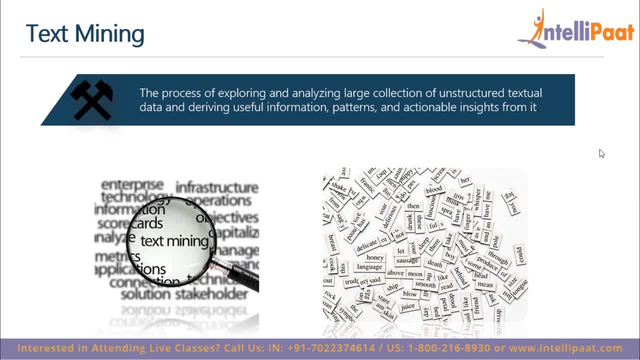 the amount of dollars a stock increased over the past week, or the number of items in the past week or the number of items sold in a day. So this number 30 could mean anything, and without proper context you wouldn't get the right information. And this is where Text. 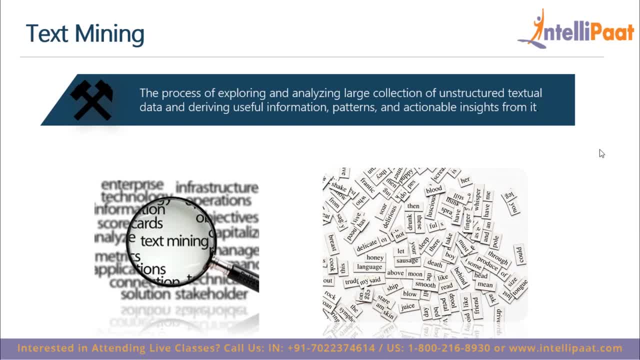 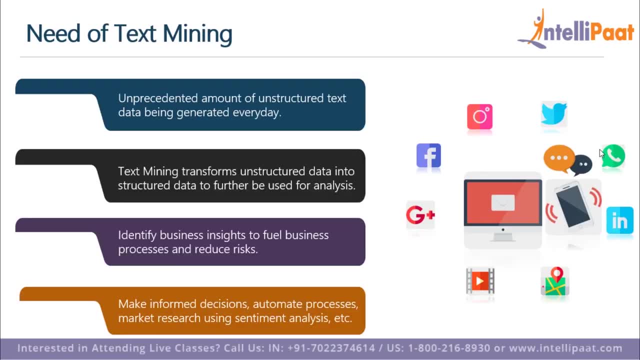 mining comes in. So, with the help of Text mining, we can give proper context to the words before and after the number 30, and this would help us to find out more information. Now let's look at the need of Text mining. So today, with the advent of social media, 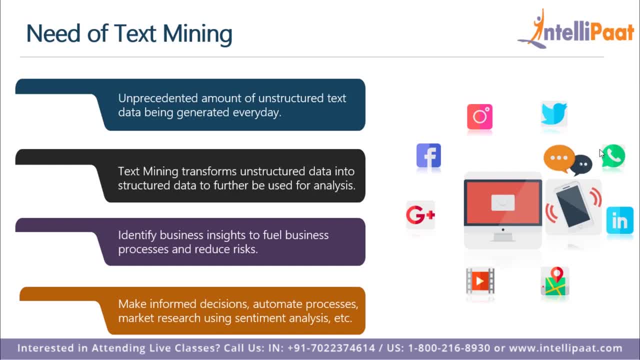 companies now have access to massive behavioural data of their customers, and most of this data is present in the phone form of unstructured textual data. But beneath this textual data lies an enriching source of information which can help companies to boost their business, And this is the reason why text 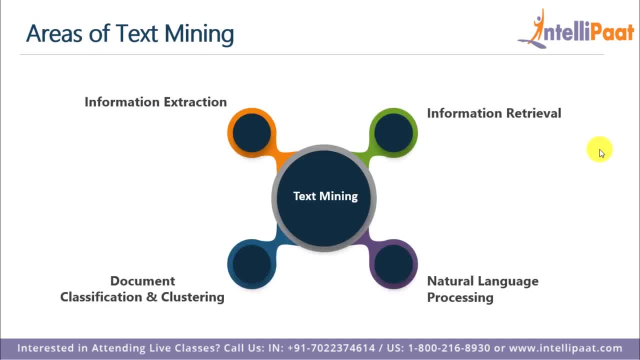 mining is being used across various industries. Now, text mining can be divided into four practice areas. So we've got information extraction, which basically deals with identification and extraction of relevant facts and relationships from unstructured data. Then we have document classification and clustering, which aims at grouping and categorizing terms, paragraphs. 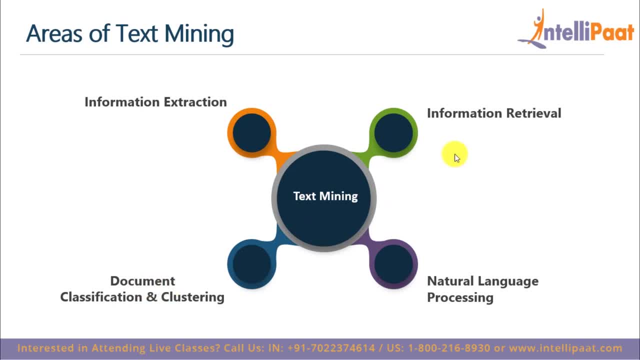 or documents using classification and clustering methods. After that we have information retrieval, which aims at storage and retrieval of text documents, And then we have NLP, which forms the major part of text mining. So here we use different computational tasks to analyze and 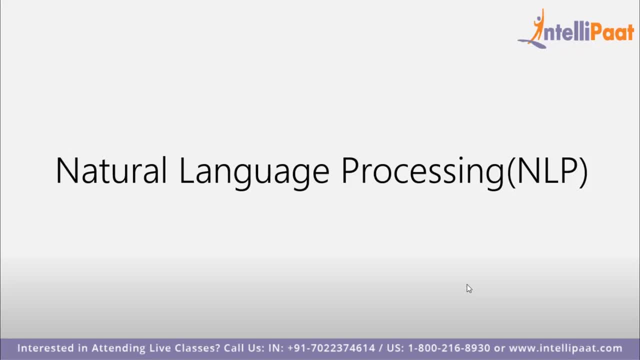 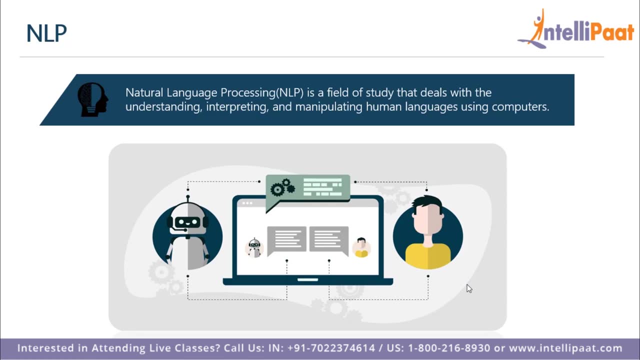 understand the underlying structure of text. So this is the first part of text: mining the text data. right now we'll dive into NLP. so when you hear the term natural language processing, the first question to pop into your head would be: what is a natural language? so any language that is used for communication by humans is. 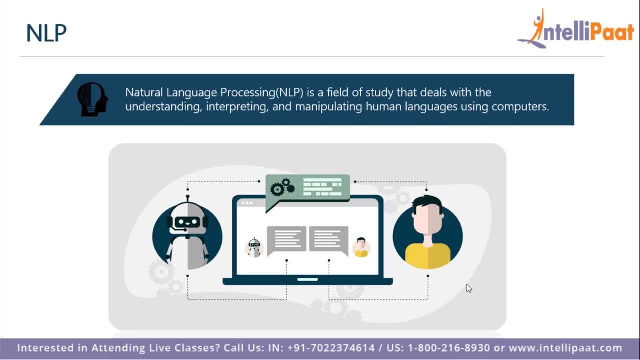 known as natural language. so English, French, Chinese, all of these are natural languages. now, since we are humans, they're able to understand these languages. but what about a machine? how is a machine able to comprehend all these human spoken languages? well, this is where NLP comes in, so natural. 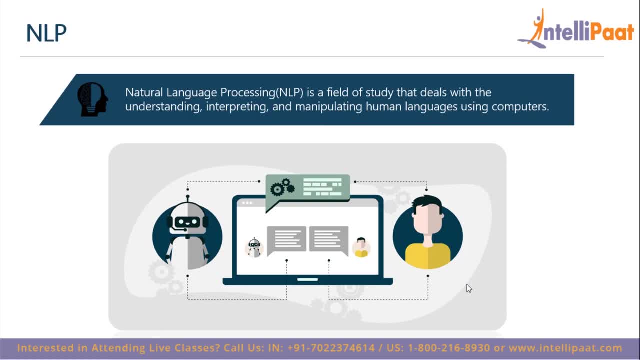 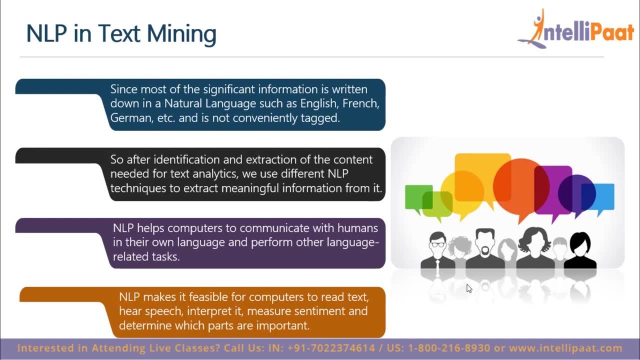 language processing is a subdomain of artificial intelligence, where we understand and interpret human languages using a computer. now let's see how is NLP used in text mining. so just think about how much text you see each day: email, SMS, web pages, the list is just endless. so with the help of NLP, we can. 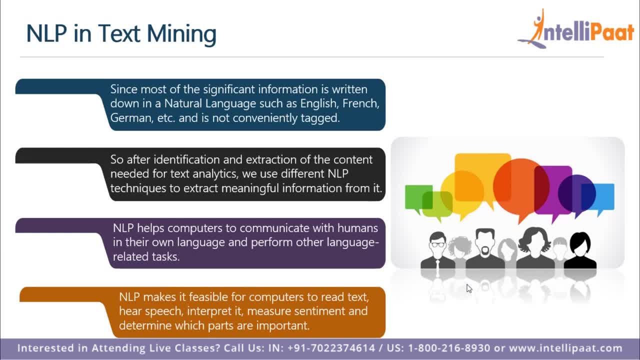 go through all of this text data and use it for different purposes. you can go through all of this text data and use it for different purposes. so, with the help of NLP, we can go through all of this text data and use it for different purposes, such as character recognition, sentiment analysis and spell checking. right now, 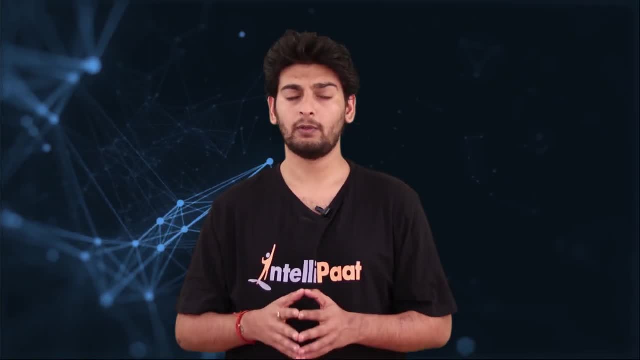 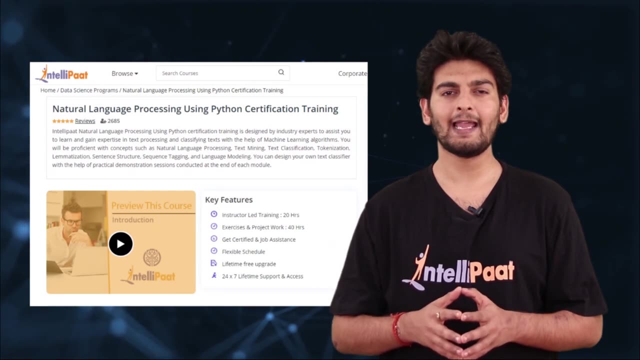 we'll go ahead and install anaconda into our systems, right guys? so just a quick info. if you are interested in doing an end-to-end certification in NLP, then Intellipaat provides the natural language processing training course. so you can check out the course details in the description below. so let's continue. 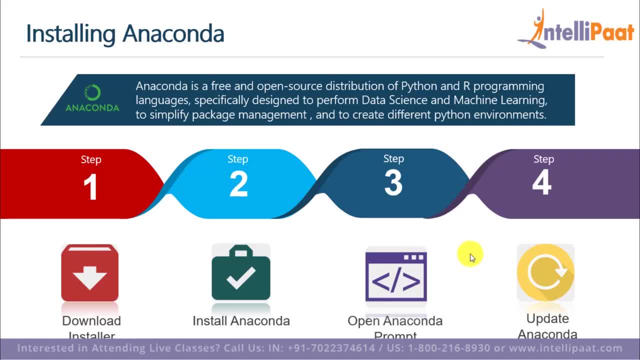 with the class. so anaconda is basically your free and open source distribution for Python and our programming languages, and it is specifically designed to perform data science and machine learning applications. right? so these are the four steps to work with anaconda. so first we have to download the 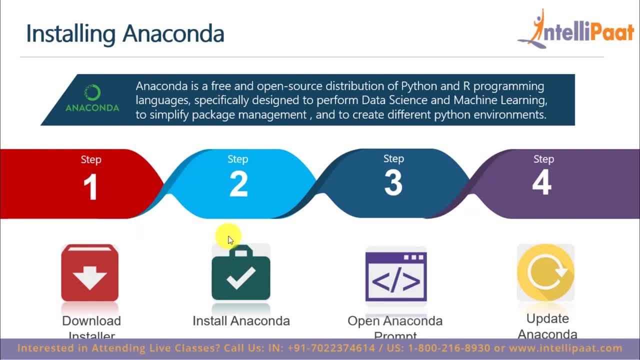 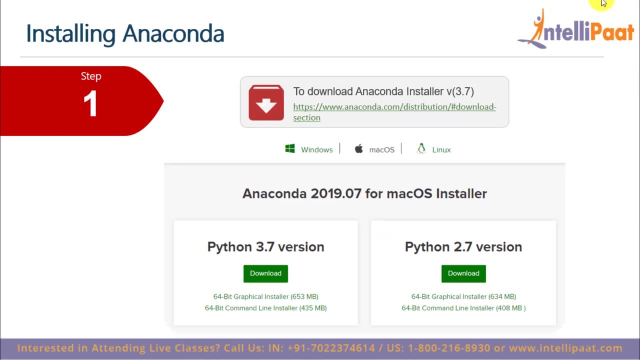 anaconda installer and then we'll install anaconda. then we'd have to open anaconda prompt and update anaconda right now. let me just guide you how we can do this. so first we'd have to go to this website, anacondacom distribution download section, and you'd have to download the version for whichever. 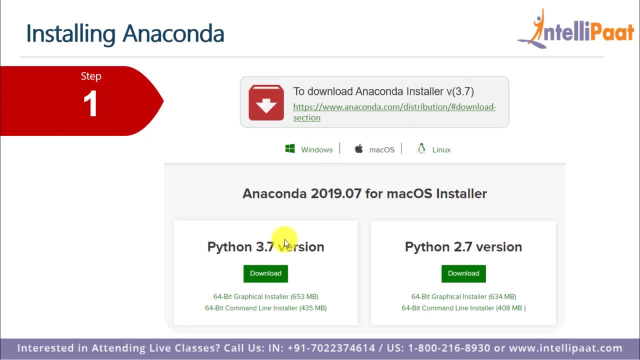 operating system you're using. so if you're using a Windows system, then you'll download anaconda for Windows, and then you'll have to download the version for Windows. if you're using Mac, then you'll download it for Mac, and if you're using Linux, then you'll download it for Linux. now you've got two versions of Python, so 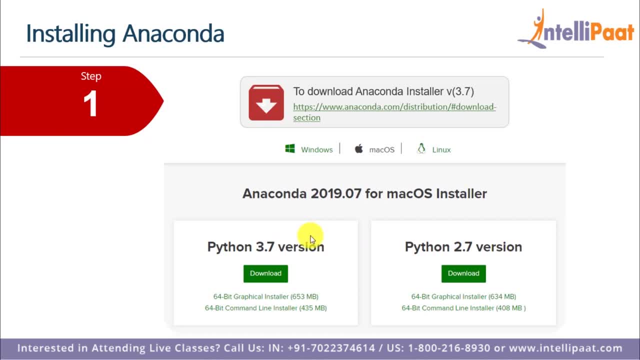 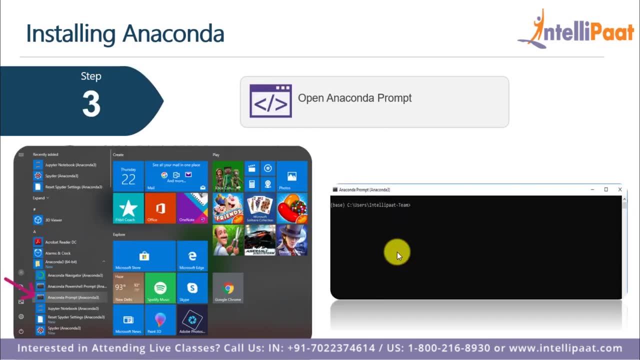 Python 3.7 and Python 2.7, and we'll be downloading the latest version of Python, which is Python 3.7. so once we download this, we have this setup wizard over here, so we just have to click on next and it'll take care. now, once the installation. 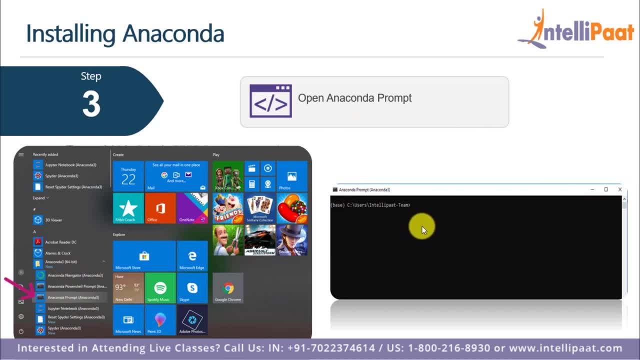 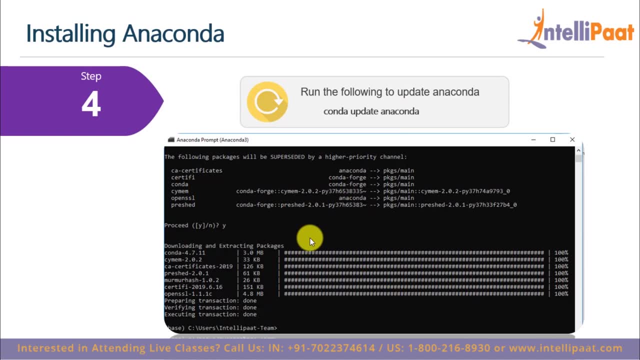 is done, we'd have to open up the command prompt. so this is what we get when we open the anaconda prompt. now, inside this we'd have to type in conda, update anaconda and we'll have the latest version of anaconda in our system. all right, now let 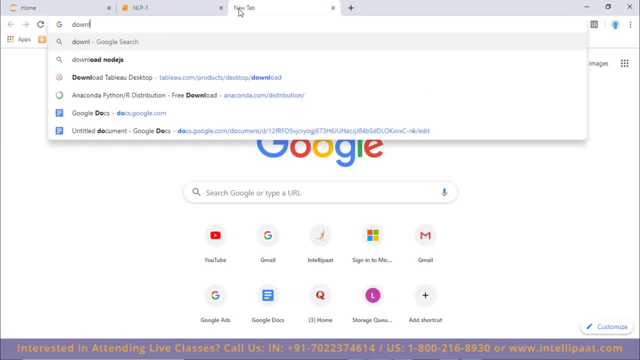 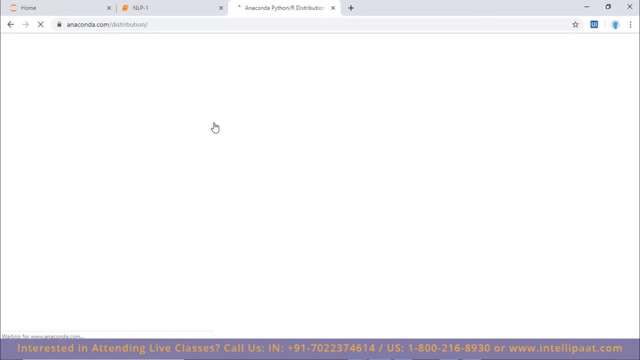 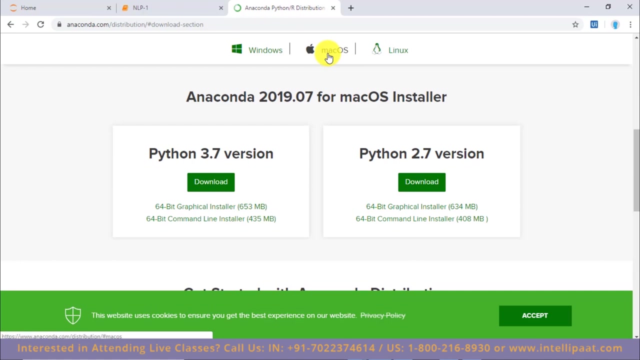 me just go ahead and show how to do it. so I'll just type in: download- anaconda- I'll click on this link over here, and anaconda python r distribution, and over here I'll click on this download. so I've got different, doesn't? oh, here for 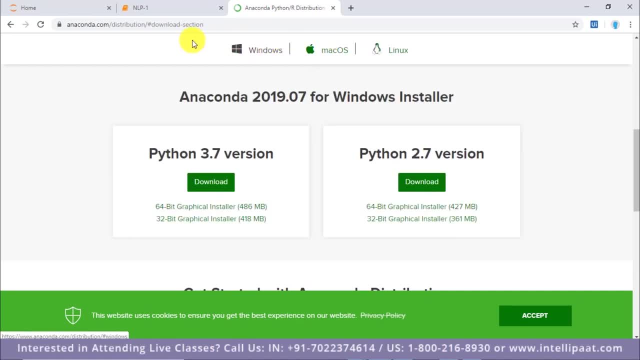 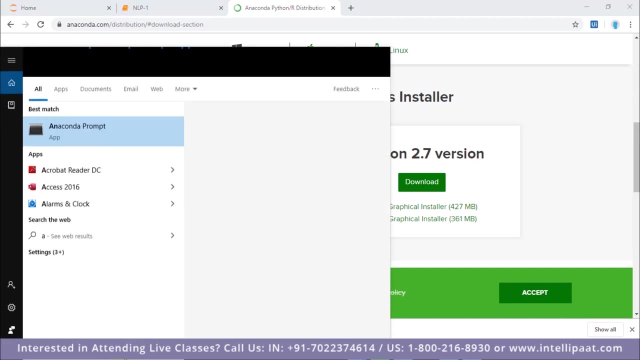 Windows, Mac and Linux and since I'm using a Windows system, I'll download anaconda for the che v LinkedIn Windows system. so this is the latest version of Anaconda Python 3.7. I just have to click on download right. so once the download is done, I'll get a setup wizard and I'd have to set it up and I'll go and click. 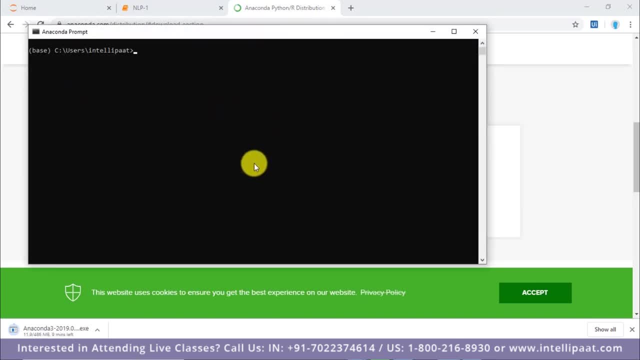 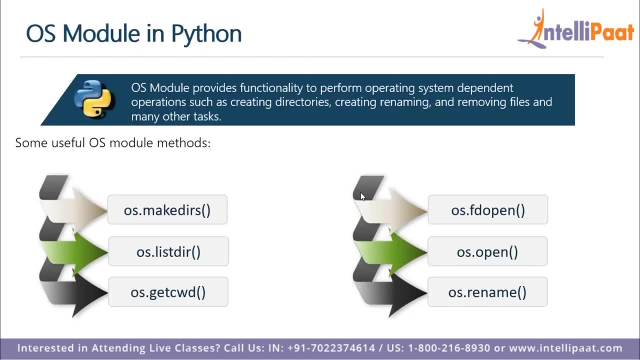 on Anaconda prompt. so this is my Anaconda prompt over here. so now that we've successfully installed Anaconda into our systems, we'll go ahead and work with the OS module. right? so the OS module: it provides functionalities to perform operating system dependent operations. so these operations include: 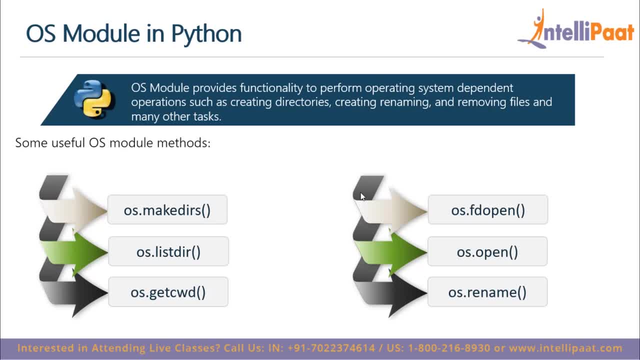 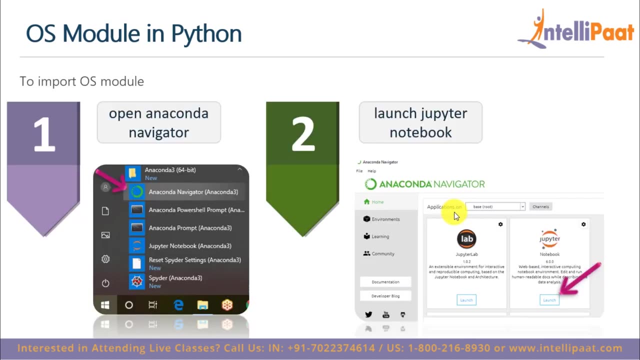 creating directories, creating, renaming and removing files and many other tasks. and these are the different methods we've got. so we've got OS dot rename, OS dot open, OS dot list directory, OS dot make direct, OS dot get current working directory and OS dot FD open. now to work with the OS library we'll have to launch. 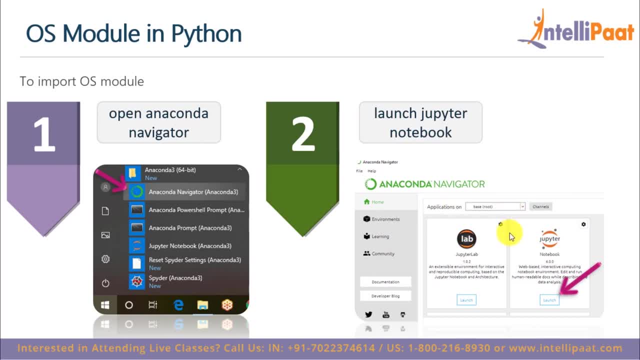 the Jupyter notebook. so we can either launch the Jupyter notebook through Anaconda navigator or we can launch it through the Anaconda prompt. so Anaconda navigator basically provides you a GUI and then we can launch it through the Anaconda prompt and then we can launch it. 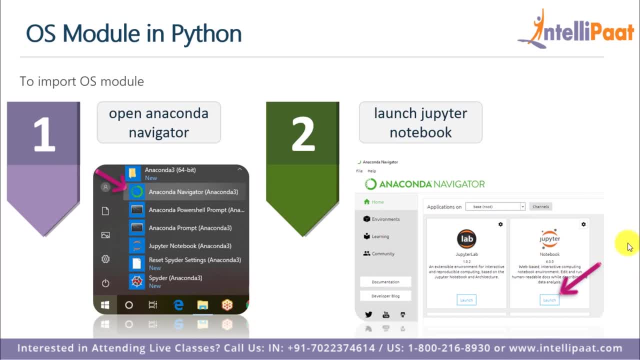 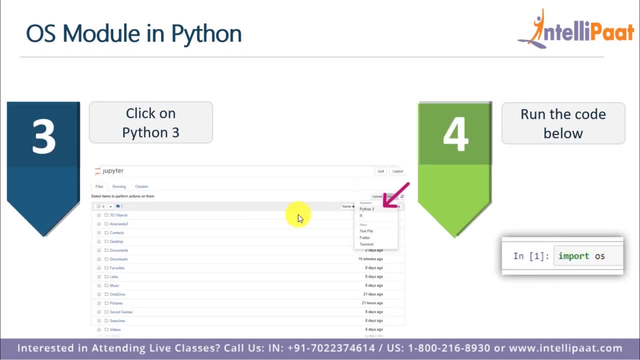 through the Anaconda navigator. so you can either use this or the Anaconda prompt. now, when you open the Anaconda navigator, you have Jupiter notebook inside this and all you have to do is click on launch now. once you do that, you have your Jupyter notebook right in front of you. so over here you would have. 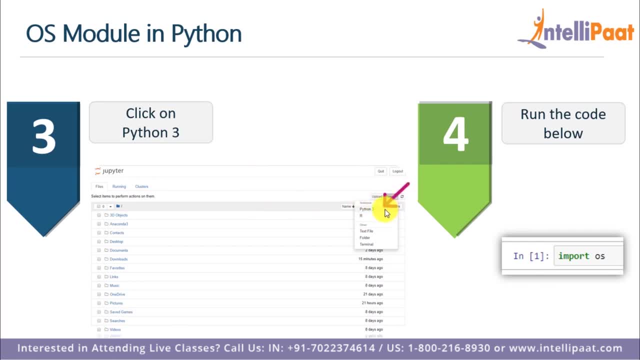 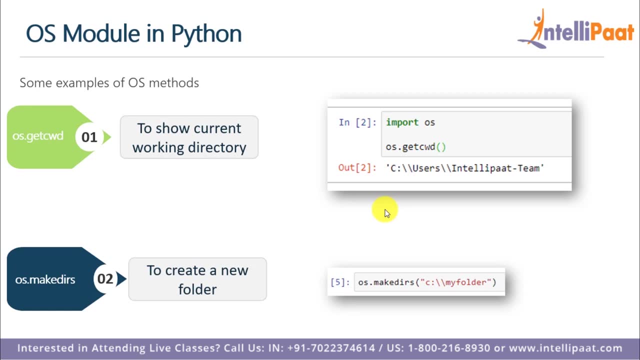 to click on new and open up a new Python notebook. now, once you do that, you have a new page and over there you'll be performing different operations. so your first task would be to import the OS library. so we'll just type in import OS. Now, if you want to have a glance at the current working system of theiverhk, 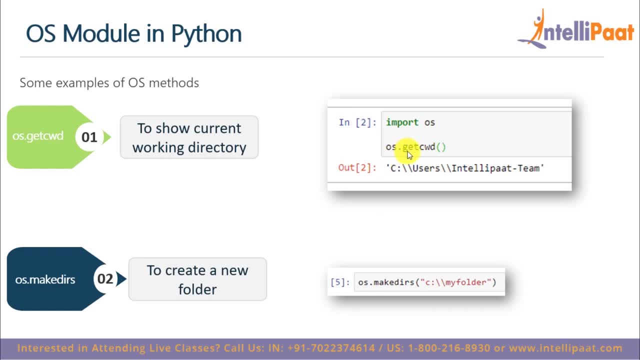 directory. all you have to do is type in os dot- get current working directory and it will give you the current working directory. and if you want to create a new folder, then you will type in os dot- make dirs and then you will give in the path. after that you will give in the name of the. 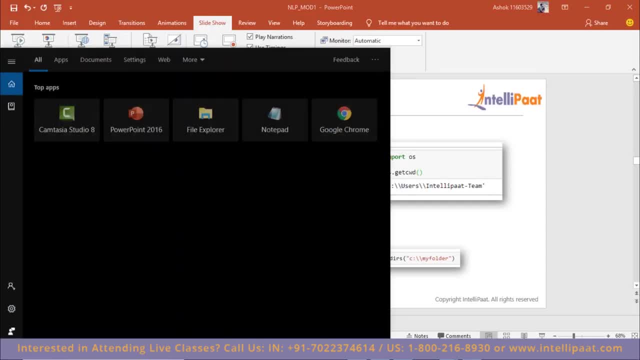 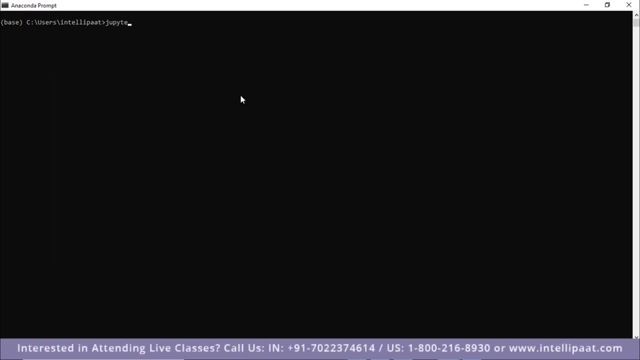 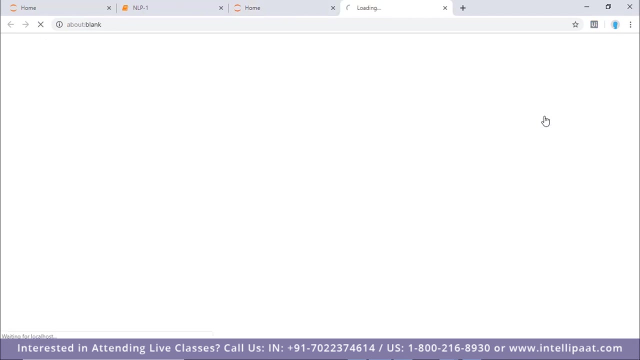 directory which you want to create. so let's perform this. so again, i'll just type in anaconda prompt over here now. inside this i'll type in jupyter notebook right. so now we see that we've launched the jupyter notebook over here. now i'll click on new and i'll open up a new python 3. 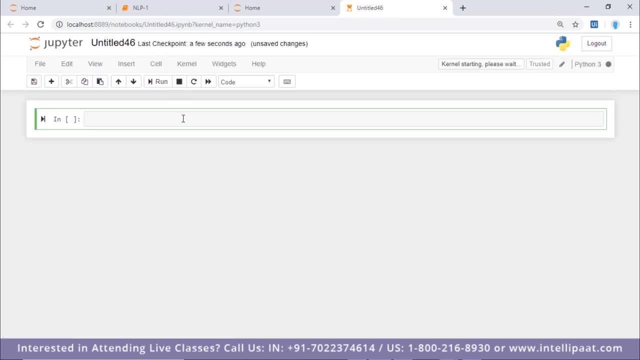 notebook. so our first task was to import the os module. so i'll type import os and i've successfully imported this module. so, as i stated in the ppt, the os module is basically used to work with different operating system applications. so you can create different directories you can open up. 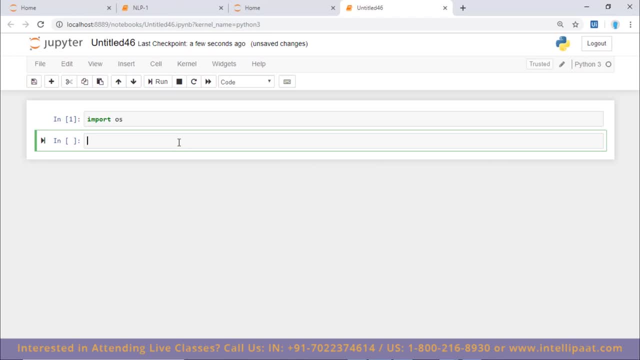 new files, you can rename files and so on. so our first task over here is to have a glance at our current working directory. so i'll type in os, dot, get cwd and i'll put in the parenthesis over here: right? so this is my current working directory c. 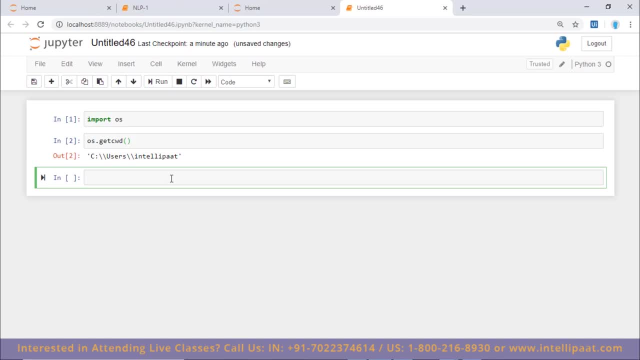 uses intellipath. now i want to make a new directory in my c drive, so this would be the command for that. so i'll type in os dot, make dirs, and over here i'd have to give in the path. so i'll type in c colon, double slash and i. 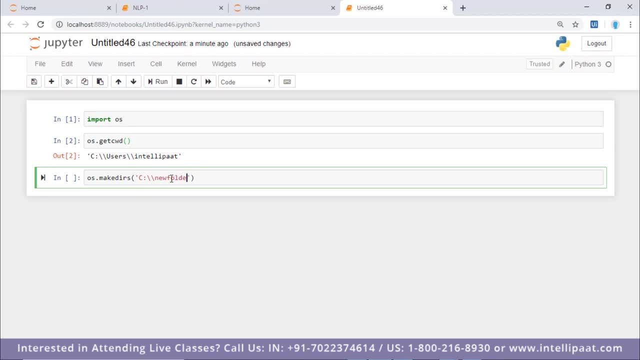 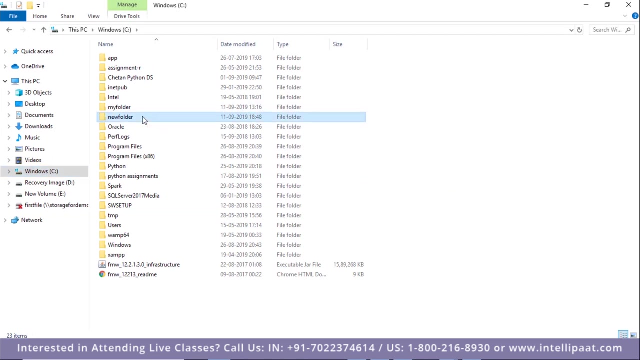 name the folder as, let's say, new folder. let me click on run right. so now i've successfully created this folder. now let me actually go to the c drive and see if this folder exists or not. so this is my c drive over here and i see that we have this folder with the name. 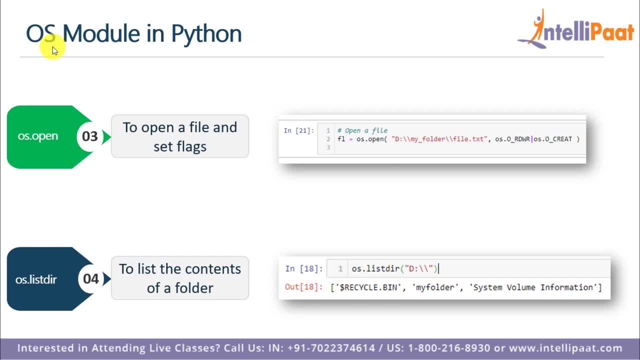 new folder. now we'll go ahead and perform some more operations. so let's say i want to open a file which is present in my system. so to do that i've got this command os dot open and inside this i will give in the path of the file and then i'll give the name of the. 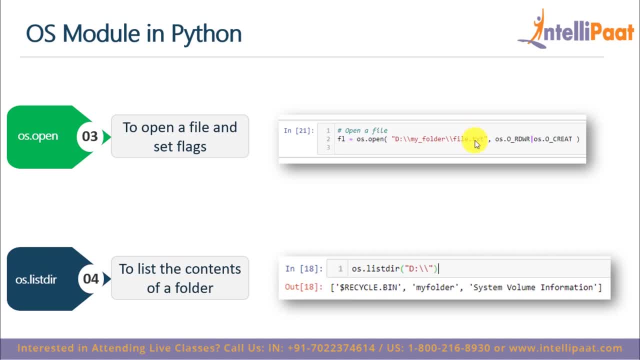 file. after that i also have to give the extension of file right. so this is a text file. so i'll type in file dot text and over here this is basically the flag. so so over here i'd basically be setting what sort of operation i want to do. so o underscore rdwr, it stands for read and write. so i've got. 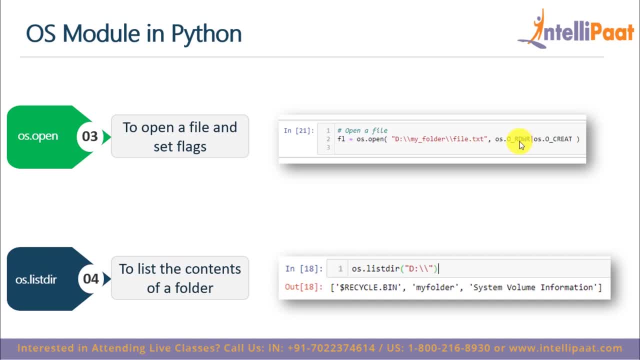 different operations. so i can open this file in only either read format or write format or read format. now, after that we set in another file. so let's say i want to open this file and i'll type in another parameter over here, which is os, dot o underscore create. so this means that if a file 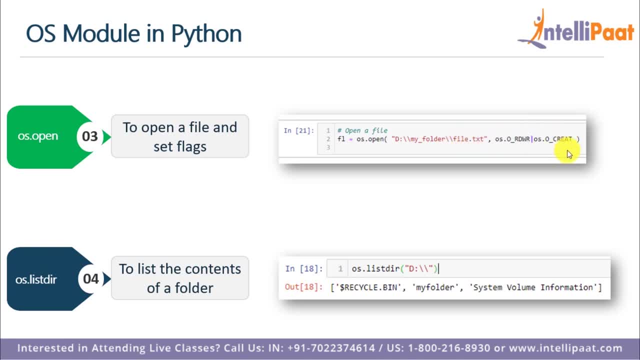 with the name file dot txt doesn't exist, then it'll automatically create this new file and then it'll open it up, and then we've got another operation. so if i want to have a glance at all of the contents which are present in a folder, then for that the command would be os dot list. 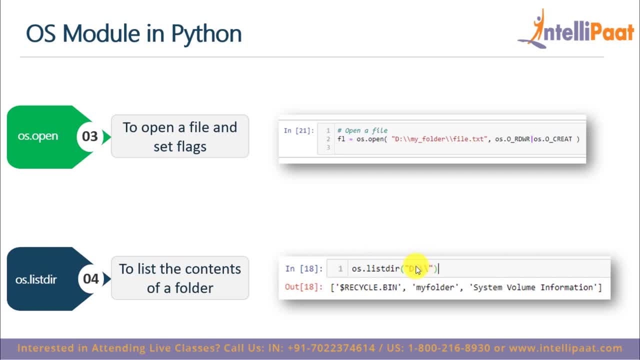 and i will give in the path. so over here, i want to have a glance at all of the contents which are present in the d drive, so i'll just give in d over here. so these are all of the contents which are present in the d drive, right so now. 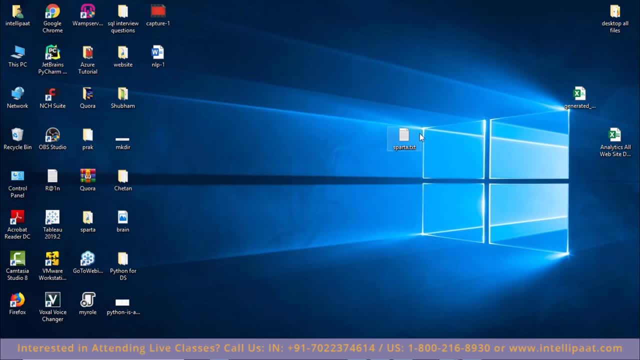 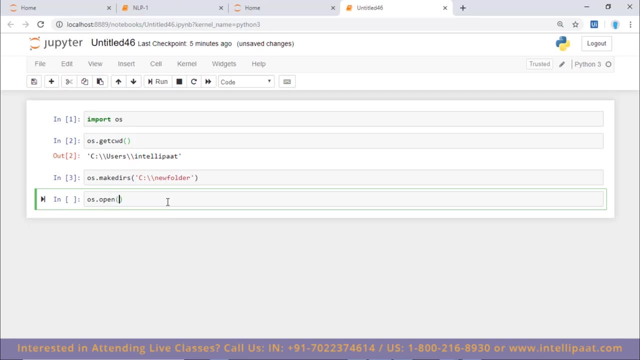 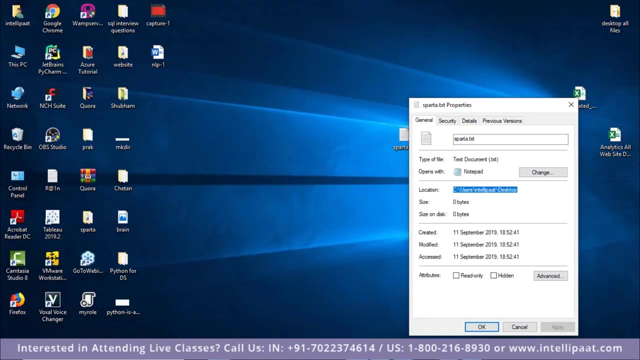 i'd want to open this sparta dot txt file using the os module, so let me do that. so the command was os dot open and inside this, as we saw first, we'd have to give in the path. so let me copy the path over here. i'll click on properties, i'll copy all of this and i'll paste it over here. you'd have. 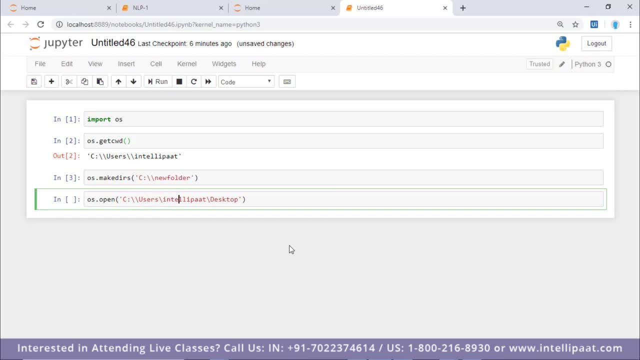 to keep in mind that you'd have to give in double slash over here, so the path over here. so to separate all of these, you'd have to give in a double slash again. you'll give in a double slash over here and then you will give in the name of the file. so the name of the file is sparta dot. 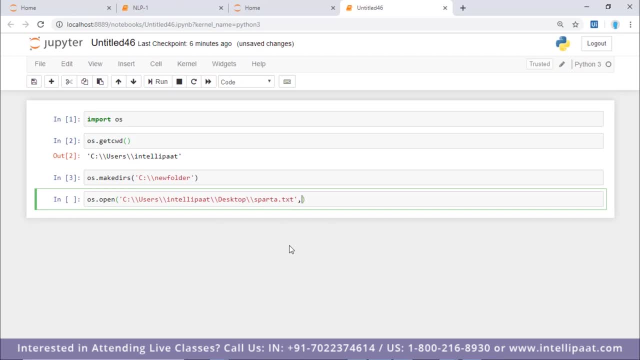 txt. after this i'll give in the flag over here, which would be os, dot o underscore. it'll be read and write and then i'll give in the pipe operator. so over here i'll just state: if the file doesn't exist, then i'll tell the operating system to create it. so 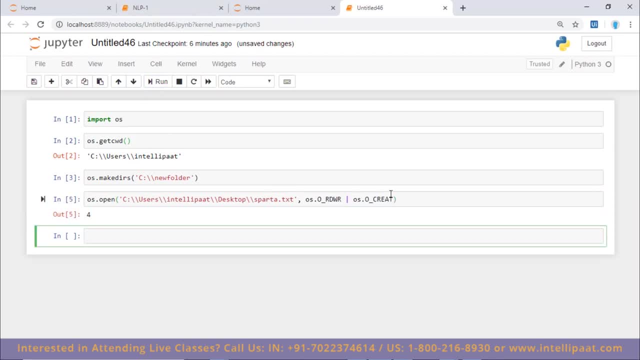 create. i'll click on run right. so we have successfully opened this file. now i'd want to have a glance at all of the contents which are present in the c drive. so i'll type in os dot list directory, and inside this i'd have to give in the path. so i'd want to have a glance at all. 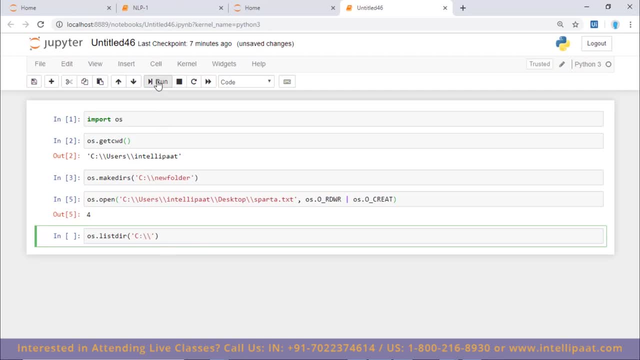 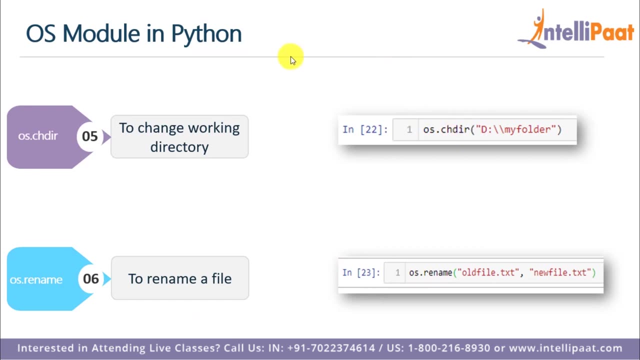 of the contents which are present in the c drive, right? so these are all of the folders, or all of the contents which are present inside the c drive. then i have a couple more commands over here. so this is the command to change the working directory. so over here i'm changing my working directory from d drive to my folder. so i just have to. 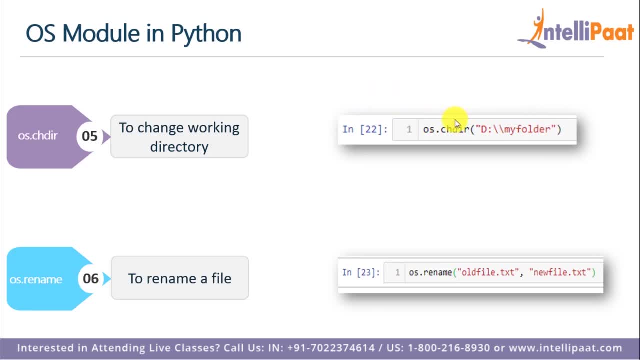 given the path for this and this is how i can change the current working directory, and then we can also change the name of a file. so let's say, if the name of the file was old file dot txt, then to rename it i'll just give in new file dot txt over here. so let's perform both of these. 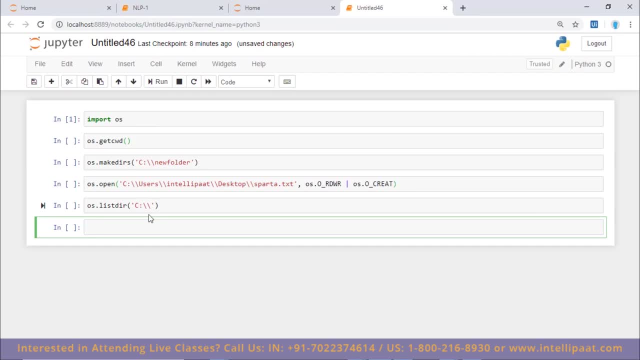 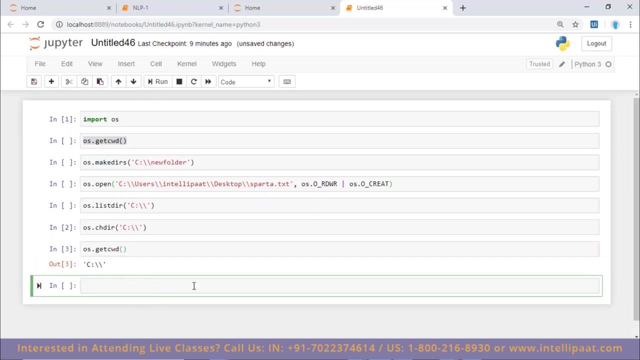 operations. so let me perform both of these operations over here. so i'll type in os dot ch, dir and inside this i'll set the working directory to c drive. c colon, double slash. right, i have changed the working directory. now let me also check the current working directory now. right, so now i have changed the working directory to c drive. 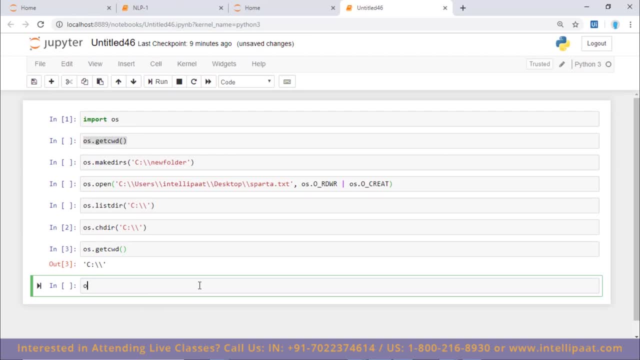 now let me go ahead and rename a file over here. so, os dot, i'll type in rename so over here. this takes in two parameters. first is the path where the file is located and the name of the file. so i'd just rename this file over here, sparta. 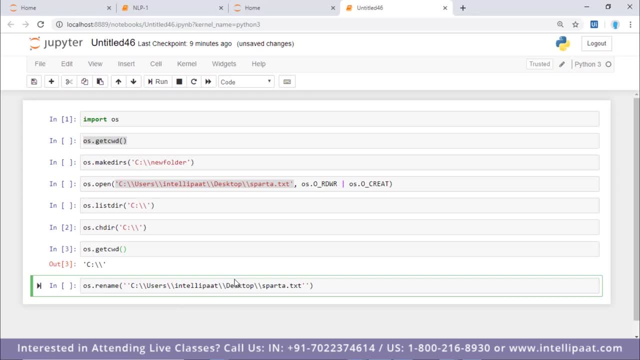 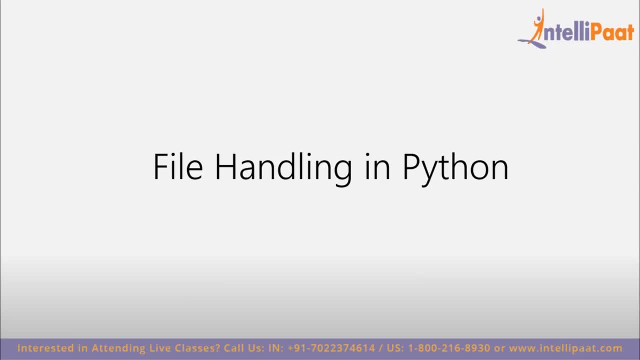 over here. so initially it was sparta dot over here. so initially it was sparta dot txt. now we've changed it to sparta new txt. now we've changed it to sparta new txt. now we've changed it to sparta new right. so that was the os module, so the os. 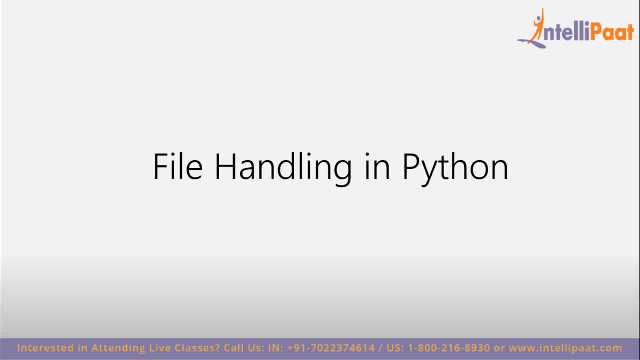 right, so that was the os module. so the os. right, so that was the os module. so the os module. we saw: how can we? we saw how can we? we saw how can we create new directories and how can we create new directories and how can we create new directories and how can we change the names of some files. now we'll. 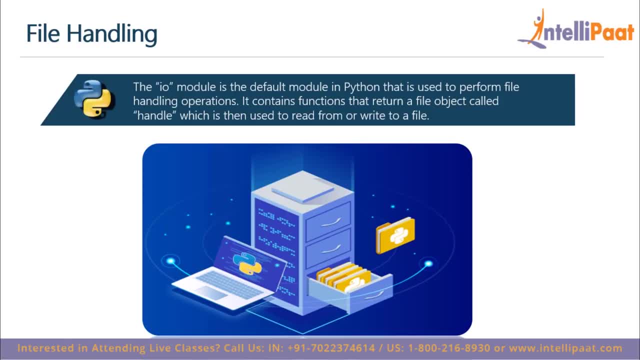 change the names of some files. now. we'll change the names of some files now. we'll go ahead and do some proper file. go ahead and do some proper file. go ahead and do some proper file handling in python. handling in python, handling in python. so the io module is the default module in. 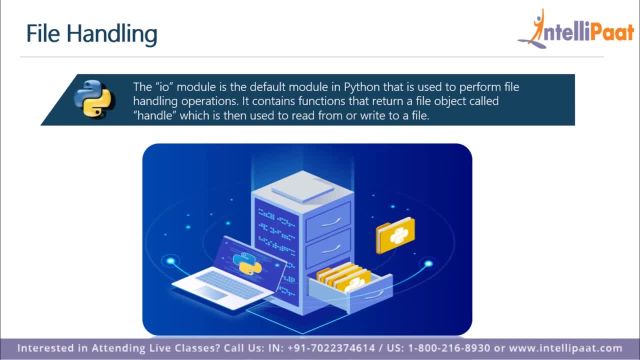 so the io module is the default module. in so the io module is the default module in python that is used to perform python. that is used to perform python that is used to perform file handling operations, and it contains file handling operations and it contains file handling operations and it contains functions that return a file object. 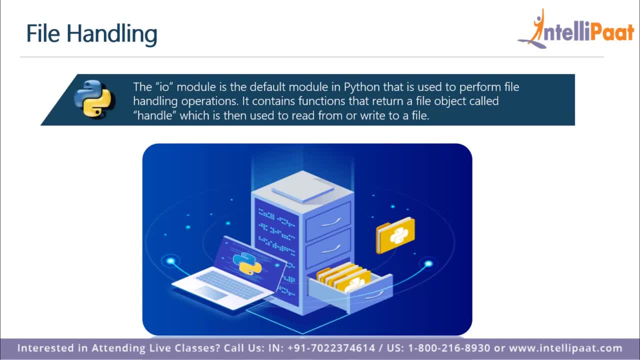 functions that return a file object. functions that return a file object called handle, and this handle is then called handle, and this handle is then called handle, and this handle is then used to read from a file or write to a. used to read from a file or write to a. 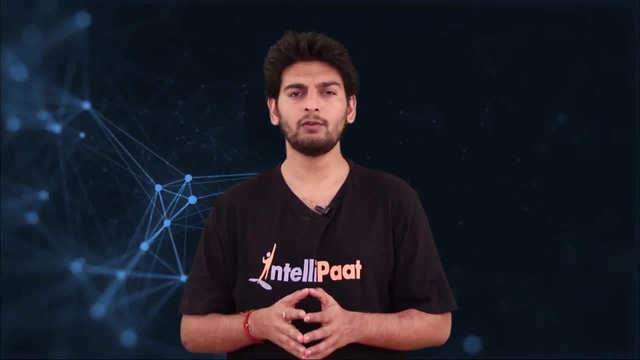 used to read from a file or write to a file, file, file, right guys? so just a quick info. if you're right guys, so just a quick info. if you're right guys, so just a quick info. if you're interested in doing an end-to-end, interested in doing an end-to-end, 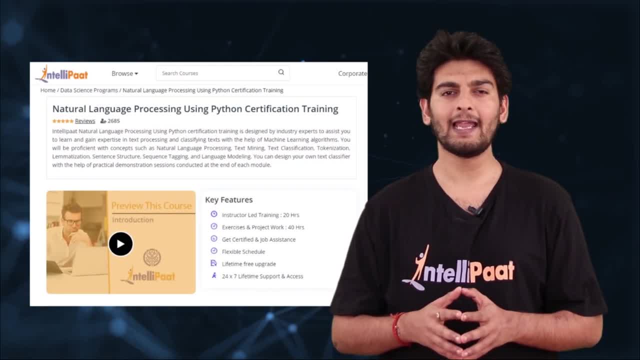 interested in doing an end-to-end certification in nlp, then intellipaat certification in nlp, then intellipaat certification in nlp, then intellipaat provides the natural language processing, provides the natural language processing, provides the natural language processing training course. so you can check out the 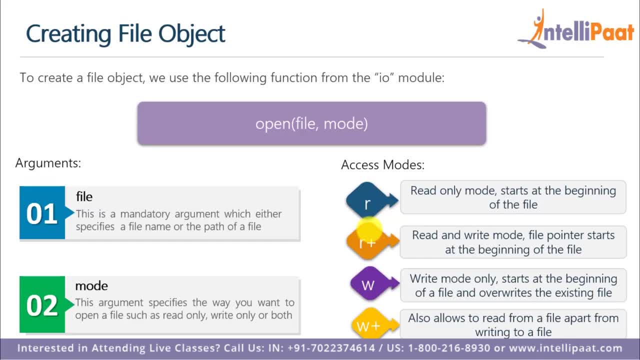 training course. so you can check out the training course. so you can check out the course details in the description below. course details in the description below. course details in the description below. so let's continue with the class so this. so let's continue with the class, so this. 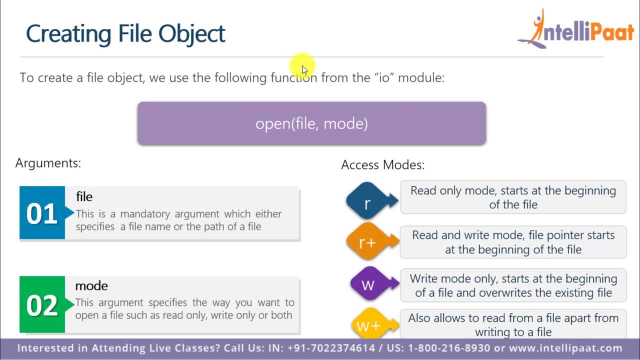 so let's continue with the class. so this is the command to create a file object. is the command to create a file object. is the command to create a file object. so we'll be using this function from the. so we'll be using this function from the. 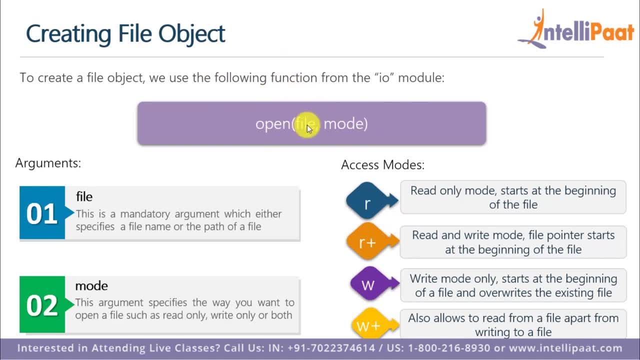 so we'll be using this function from the io module so open and this has two io module so open and this has two io module so open and this has two parameters. so this is the first parameters, so this is the first parameters, so this is the first parameter file and over here we'll give. 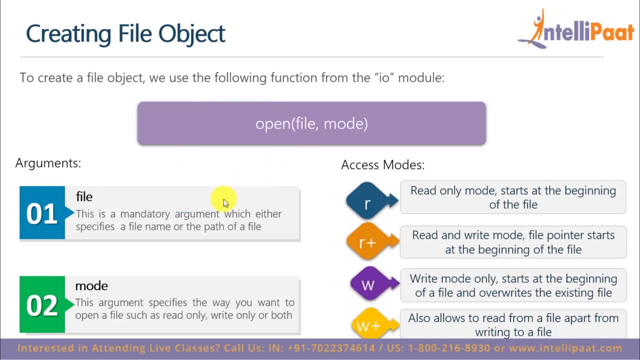 parameter file, and over here we'll give parameter file and over here we'll give in the path of the file, or just the name in the path of the file, or just the name in the path of the file, or just the name of the file. after that we've got the mode. 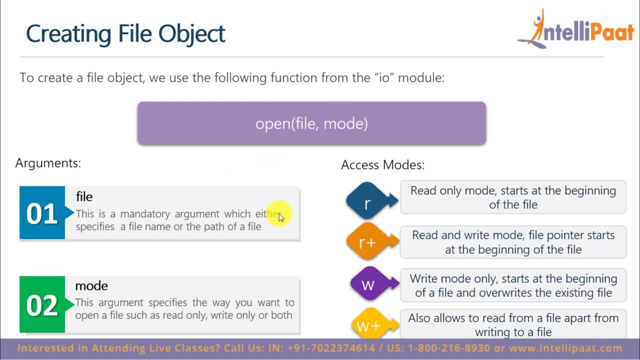 of the file. after that we've got the mode of the file. after that we've got the mode. so over here this mode. basically. so over here. this mode. basically so over here. this mode basically specifies the way we want to open a file. specifies the way we want to open a file. 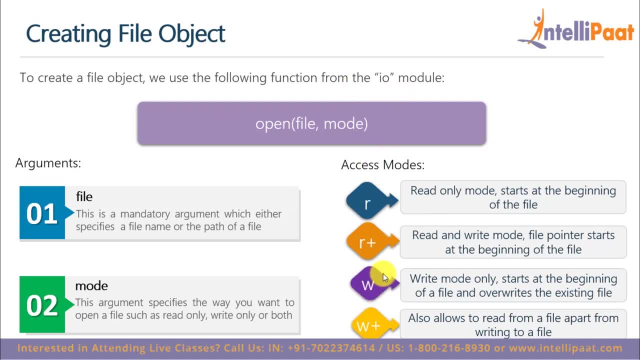 specifies the way we want to open a file. so we've got these different modes over. so we've got these different modes over. so we've got these different modes over here: r? r plus w and w plus so r. basically here r r plus w and w plus so r. basically. 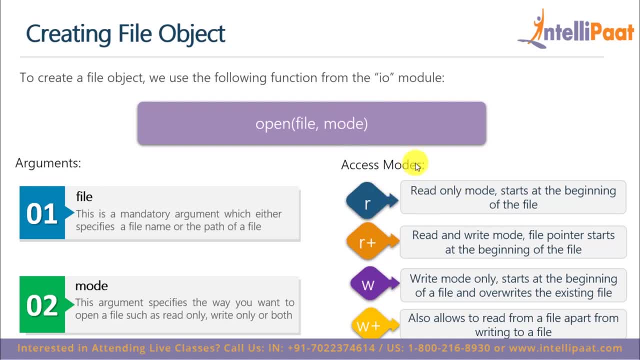 here r, r plus w and w plus so r basically stands for read only mode, right? so if we stands for read only mode, right? so if we stands for read only mode, right. so if we open a file in read only mode, then we open a file in read only mode, then we. open a file in read only mode, then we can't edit it, so it's only read only. can't edit it, so it's only read only, can't edit it, so it's only read only mode. and it starts from the beginning of mode and it starts from the beginning of. 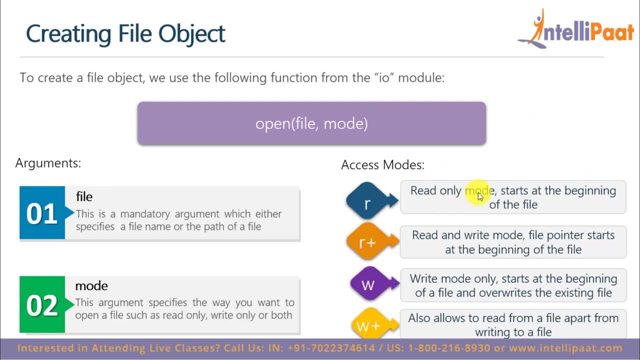 mode and it starts from the beginning of the file. after that we've got r plus the file. after that we've got r plus the file. after that we've got r plus, which stands for read and write mode. so which stands for read and write mode, so 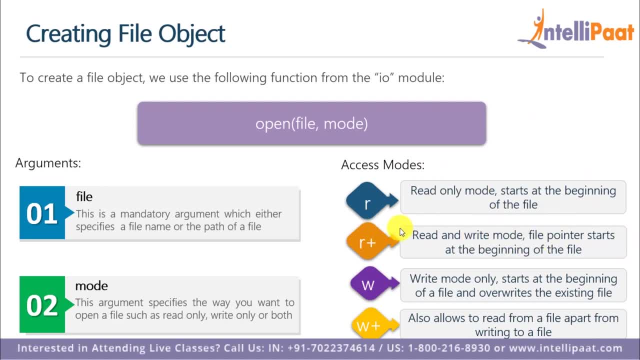 which stands for read and write mode. so over here the file pointer again starts. over here, the file pointer again starts over here the file pointer again starts at the beginning of the file and with at the beginning of the file, and with at the beginning of the file, and with this we can read the file as well as. 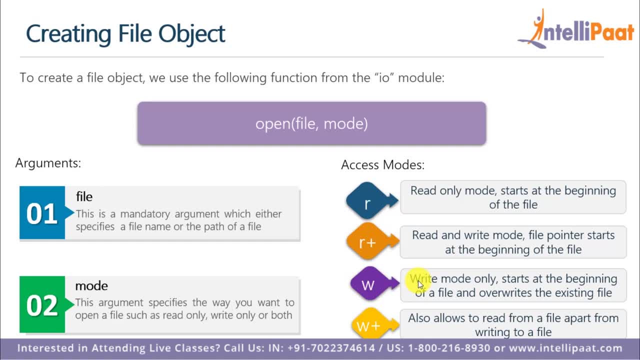 this. we can read the file as well as this. we can read the file as well as write something in the file. then we've write something in the file. then we've write something in the file. then we've got w which stands for write only mode. got w which stands for write only mode. 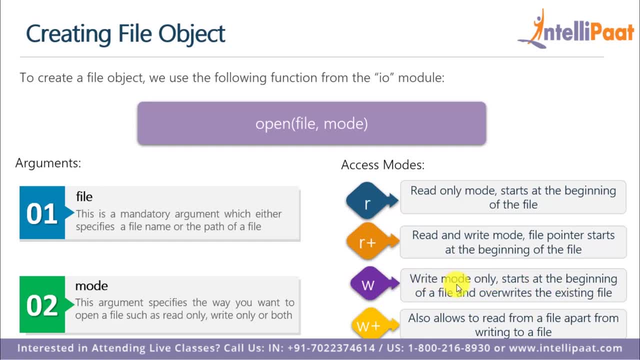 got w, which stands for write only mode. and even this, the pointer starts at the. and even this, the pointer starts at the. and even this, the pointer starts at the beginning of the file and it starts to beginning of the file. and it starts to beginning of the file and it starts to overwrite the existing file. then we've 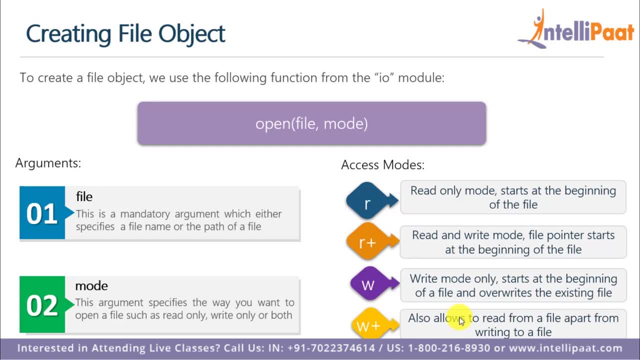 overwrite the existing file, then we've overwrite the existing file. then we've got w plus, which allows us to write, and got w plus, which allows us to write, and got w plus, which allows us to write, and as well as read. now this doesn't start- as well as read. now this doesn't start. 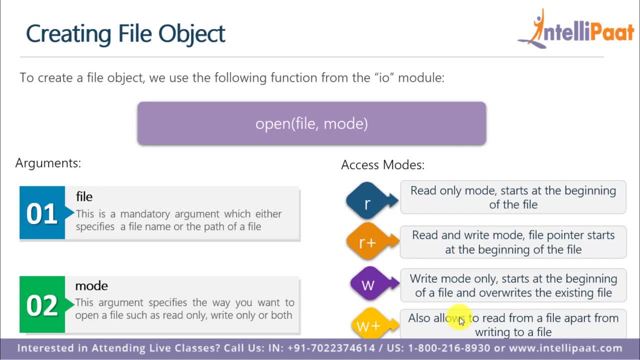 as well as read now: this doesn't start from the beginning, but it actually from the beginning, but it actually from the beginning, but it actually starts at the end of the file, right, so starts at the end of the file, right. so starts at the end of the file, right, so we can start writing from the end of the. 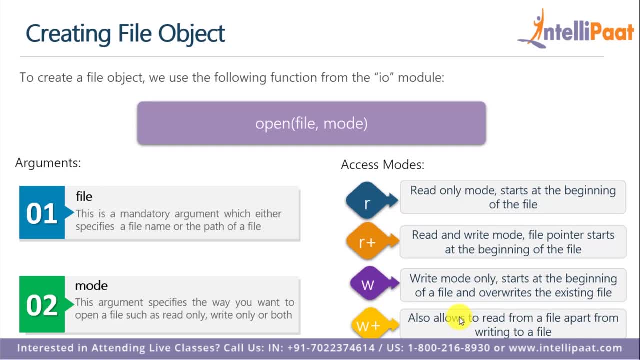 we can start writing from the end of the. we can start writing from the end of the file over here. so these are the file over here, so these are the file over here. so these are the different modes which we can open a file. different modes which we can open a file. 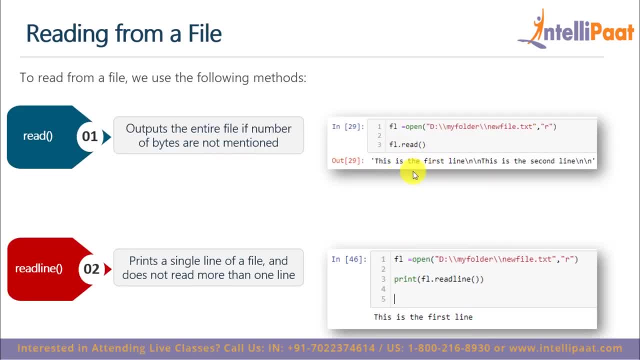 different modes which we can open a file. now, these are different methods from the now. these are different methods from the now. these are different methods from the io module with which we can read, from a io module with which we can read, from a io module with which we can read from a file. so now, let's say, we've opened up a 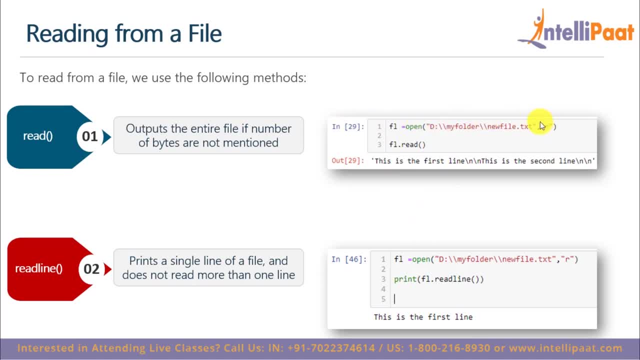 file. so now let's say we've opened up a file. so now let's say we've opened up a file so open and then i'll give in the file so open and then i'll give in the file so open and then i'll give in the path. and i'm opening this in read only. 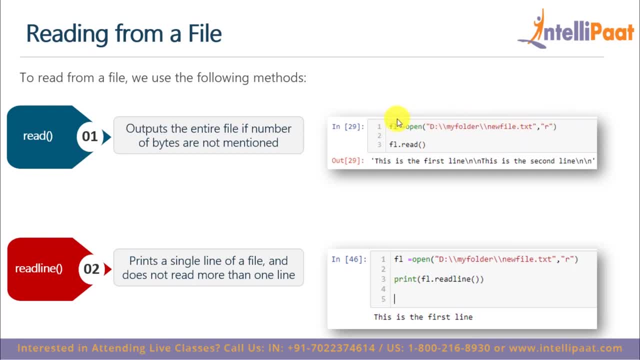 path and i'm opening this in read only path and i'm opening this in read only mode now. i'll store the file in this f1 mode now. i'll store the file in this f1 mode now. i'll store the file in this f1 instance over here now if i want to read. 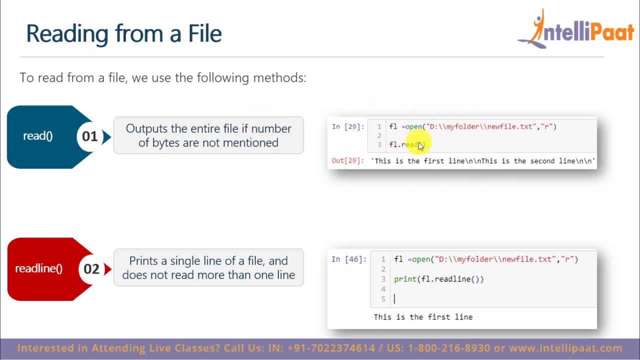 instance over here now. if i want to read instance over here now, if i want to read the entire file, i'll just type in f1 dot the entire file. i'll just type in f1 dot the entire file. i'll just type in f1 dot- read over here. so this would give me the 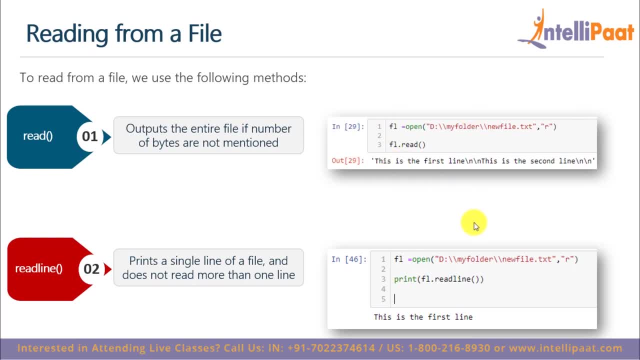 read over here. so this would give me the read over here. so this would give me the entire file over here now. instead of entire file over here now, instead of entire file over here now. instead of reading the entire file, let's say if i reading the entire file, let's say if i. 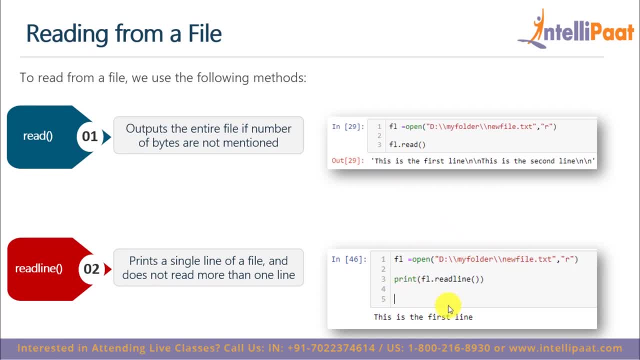 reading the entire file. let's say, if i want to read only the first line over, want to read only the first line over, want to read only the first line over there, then what i'll do is i'll type in there. then what i'll do is i'll type in. 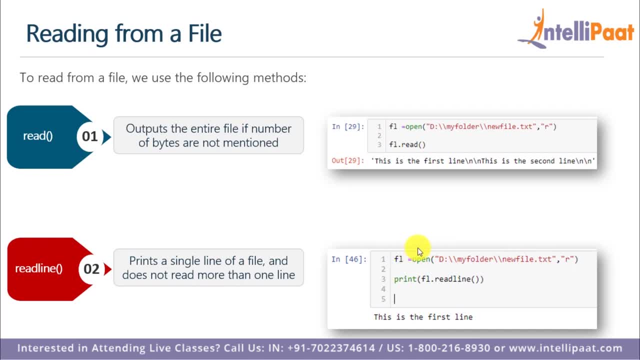 there. then what i'll do is i'll type in read line: so i'm storing this file read line. so i'm storing this file read line. so i'm storing this file. object in this f1 instance over here. object in this f1 instance over here. 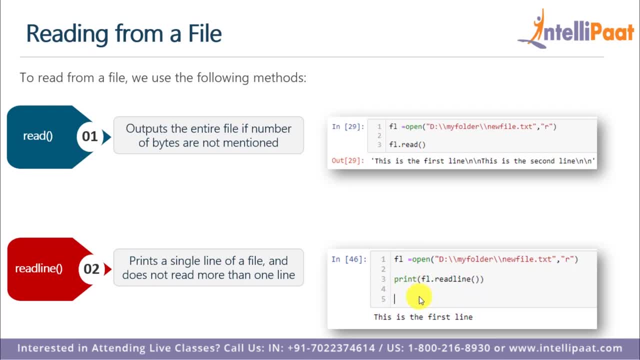 object in this f1 instance over here. after that i'll type in f1- dot read line. after that i'll type in f1- dot read line. after that i'll type in f1- dot read line, and this would just give me the first, and this would just give me the first. 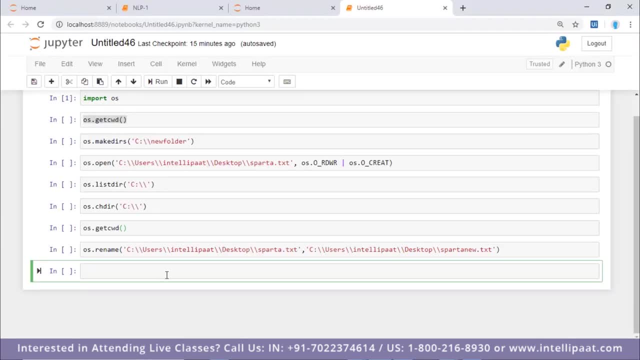 and this would just give me the first line over here. so let me perform these line over here. so let me perform these line over here. so let me perform these two operations right. so i'll type in two operations. right. so i'll type in two operations. right. so i'll type in import io over here. let me load this up. 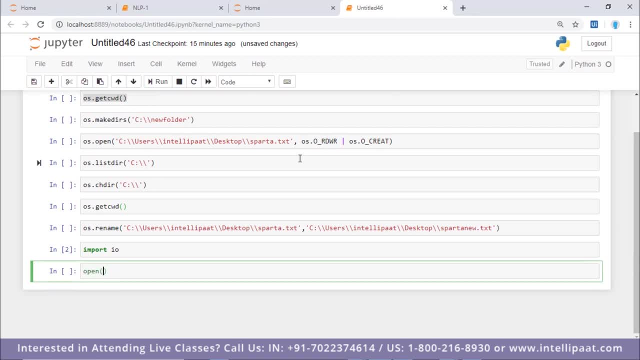 import io over here. let me load this up. import io over here. let me load this up now. i'd have to open the file, so open now. i'd have to open the file, so open now. i'd have to open the file, so open. i'll take the path. so i want to open up. 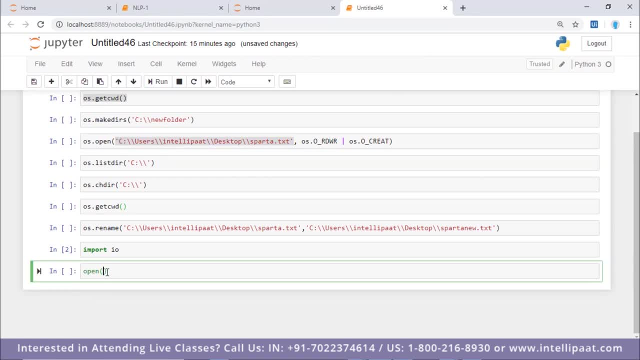 i'll take the path, so i want to open up. i'll take the path, so i want to open up the same file which is spartatxt. the same file which is spartatxt. the same file which is spartatxt. right now, i want to open this in read: 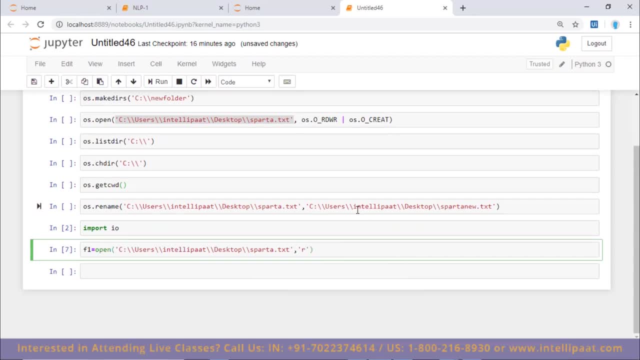 right now. i want to open this in read right now. i want to open this in read only mode. so i'll type in only mode. so i'll type in only mode. so i'll type in the contents of this file. so i'll type in the contents of this file. so i'll type in. 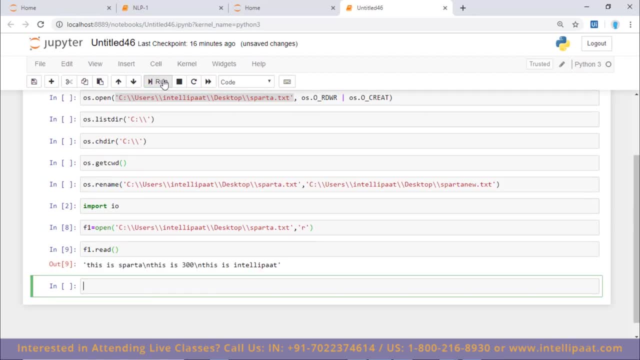 the contents of this file. so i'll type in f1.read. so these are the three lines which are. so these are the three lines which are. so these are the three lines which are present in this file. this is sparta. this present in this file. this is sparta. this. 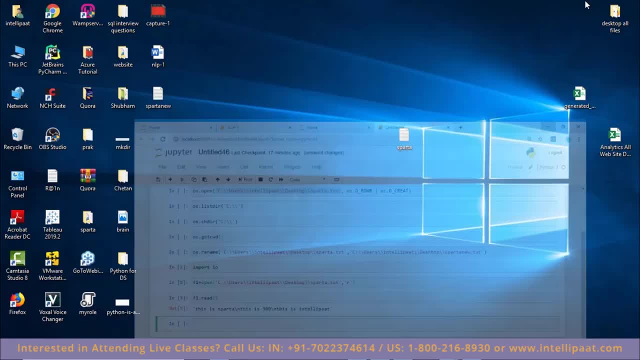 present in this file. this is sparta, this is 300 and this is intellipath. so let me is 300 and this is intellipath. so let me is 300 and this is intellipath. so let me just verify this. 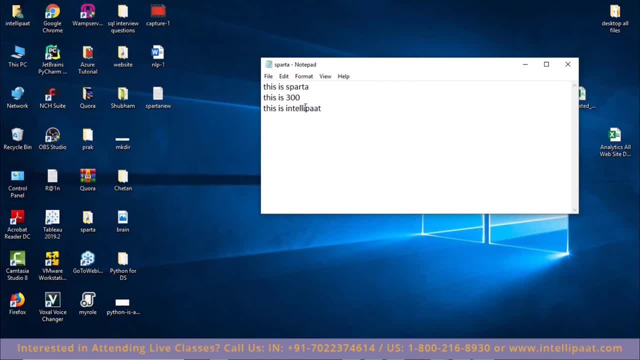 just verify this. just verify this. i'll open up this file. right, so these- i'll open up this file. right, so these? i'll open up this file. right, so these are three lines. this is part of this. is are three lines. this is part of this is. 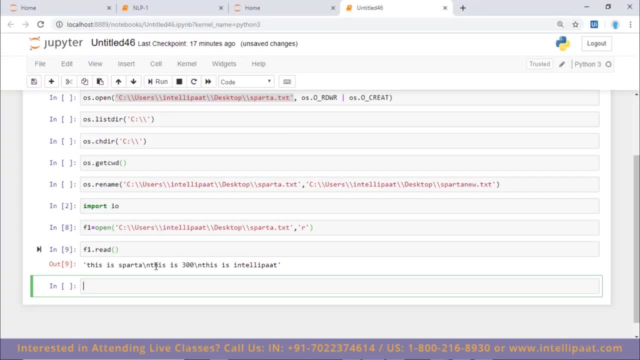 are three lines. this is part of, this is 300 and this is intellipath 300 and this is intellipath 300 and this is intellipath. now, as you see all of these three lines, now, as you see all of these three lines, 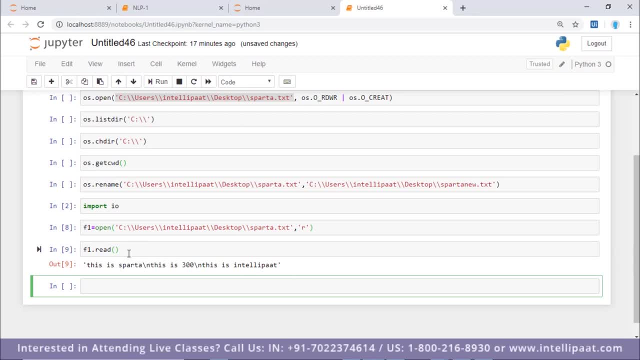 now. as you see, all of these three lines are separated by slash n. so over here are separated by slash n. so over here are separated by slash n. so over here. slash n denotes a new line, over here now. slash n denotes a new line over here now. 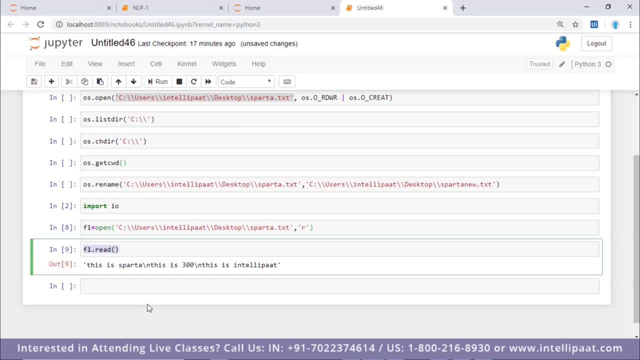 slash n denotes a new line over here. now, instead of reading all of these three, instead of reading all of these three, instead of reading all of these three lines, i want to read only the first line lines. i want to read only the first line lines. i want to read only the first line from this file. so the command for this. 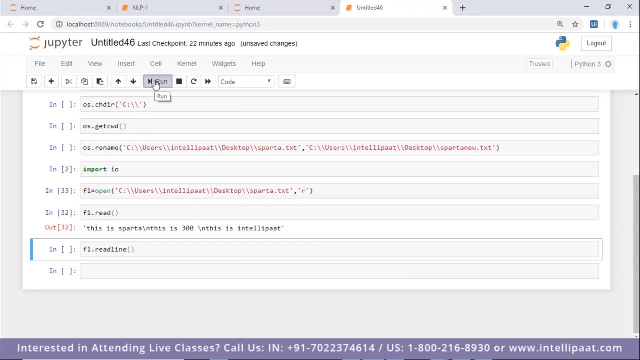 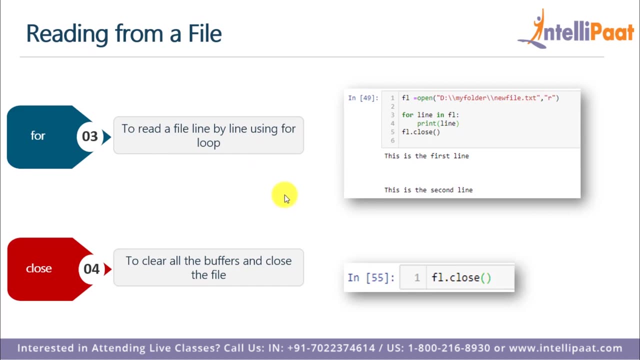 from this file, so the command for this. from this file. so the command for this would be: os dot read line right. so now would be: os dot read line right. so now would be os dot read line right. so now i can save this file in an instance. so 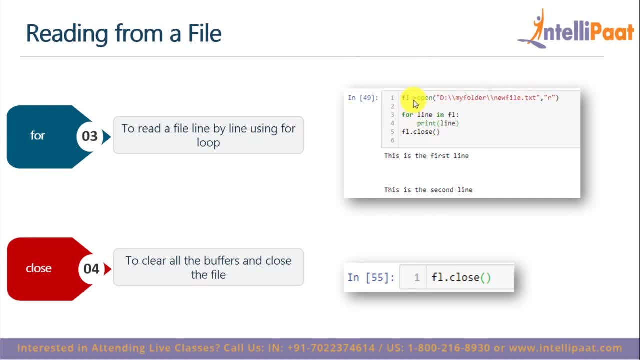 i can save this file in an instance. so i can save this file in an instance. so over here i'm saving this in f1. after over here i'm saving this in f1. after over here i'm saving this in f1. after that i'll start the for loop. so over. 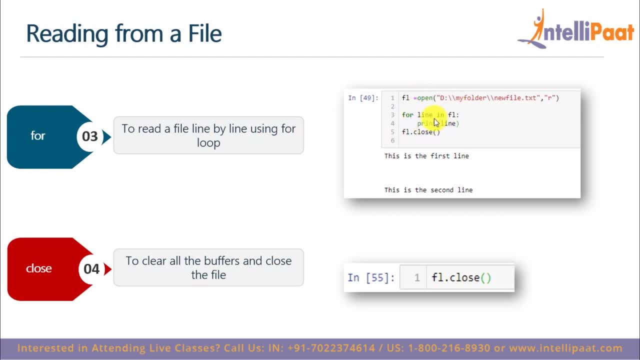 that i'll start the for loop. so over that i'll start the for loop. so over here i'll create a new variable. so for here i'll create a new variable. so for here i'll create a new variable. so for line in f1. and this line stores every. 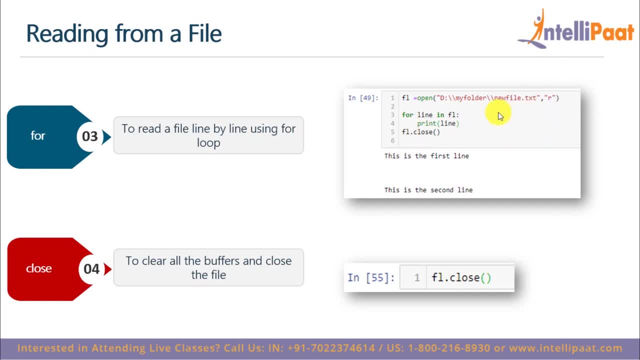 line in f1 and this line stores every line in f1 and this line stores every line which is present in this file over line which is present in this file over line which is present in this file over here. so it will store the first line and here, so it will store the first line, and here, so it will store the first line, and then we are printing the first line now. then we are printing the first line now, then we are printing the first line now. once that is done, it will go back and once that is done, it will go back. and once that is done, it will go back and then print the second line and it will then print the second line. and it will then print the second line and it will go back and then print the third line. go back and then print the third line. 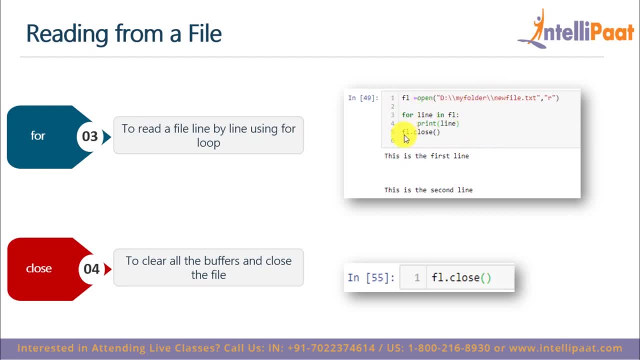 go back and then print the third line, right. so this is what happens now after right. so this is what happens now after right. so this is what happens now after we print all of the lines. i'm just we print all of the lines. i'm just we print all of the lines. i'm just typing f1 dot close. so when i type f1, 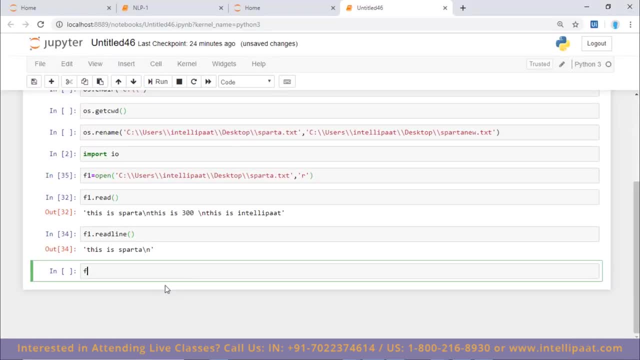 typing f1- dot close. so when i type f1, typing f1- dot close. so when i type f1, dot close, it'll just clear all of the dot close. it'll just clear all of the dot close. it'll just clear all of the buffers and close the file. so i'll just 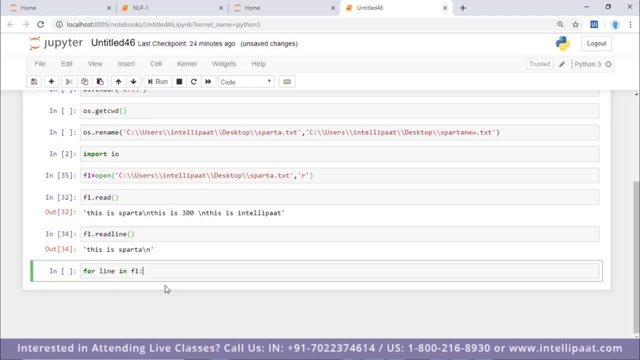 buffers and close the file. so i'll just buffers and close the file. so i'll just type in for type in for type in for line in f1 and over here line in f1 and over here line in f1 and over here i want to print f1. 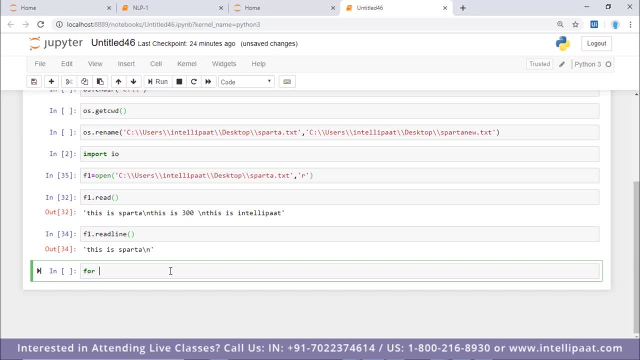 i want to print f1. i want to print f1, right. so let me start off by using the right. so let me start off by using the right. so let me start off by using the for loop. so i'll type in for for loop, so i'll type in for. 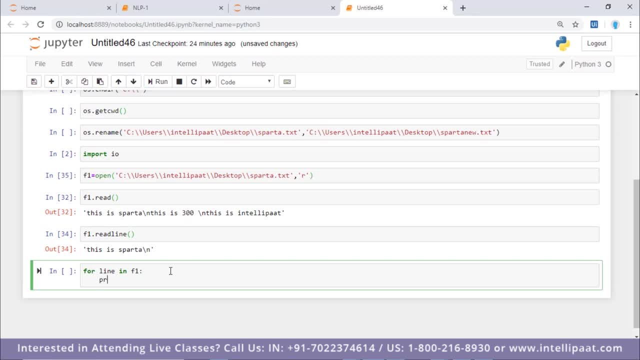 for loop. so i'll type in for line in f1 and i'd have to print each line in f1 and i'd have to print each line in f1 and i'd have to print each of the line. so i'll type print line of the line. so i'll type print line. 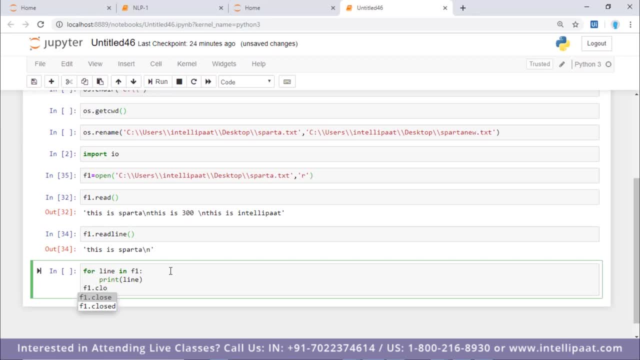 of the line. so i'll type print line and i'd have to close the buffer, so f1 and i'd have to close the buffer, so f1 and i'd have to close the buffer, so f1, dot, dot, dot, close, close, close. let me close this. 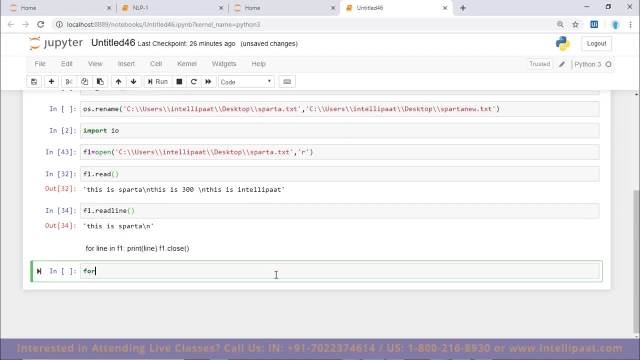 let me close this. let me close this now. let me click on run now. let me click on run now. let me click on run right. so let me start off by using the right. so let me start off by using the right. so let me start off by using the for loop over here. so i'll type in for: 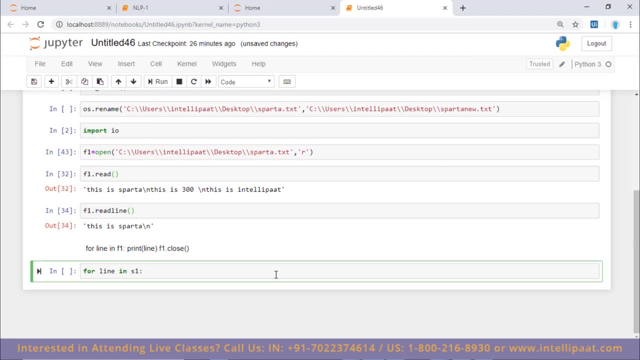 for loop over here. so i'll type in for for loop over here. so i'll type in for line in line in line in f1: f1. so this is f1 and not as one i'd have to. so this is f1 and not as one i'd have to. 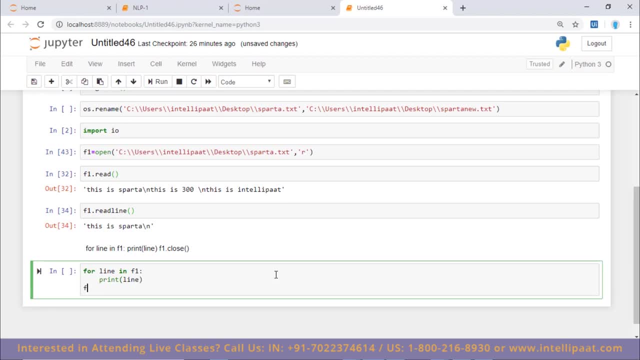 so this is f1 and not as one. i'd have to print each of the lines, so i'll type in print each of the lines. so i'll type in print each of the lines. so i'll type in print line and then i'd have to close. 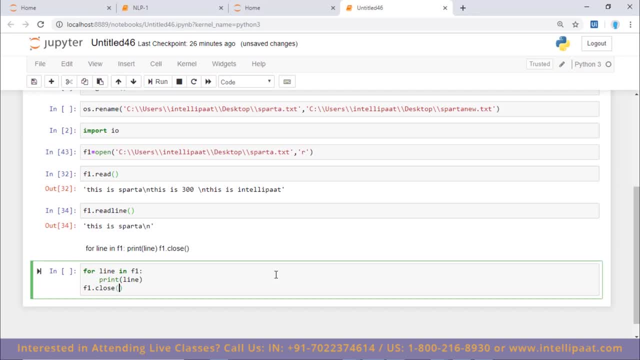 print line and then i'd have to close print line and then i'd have to close the file. so i'll type in the file, so i'll type in the file, so i'll type in: f1 dot, f1 dot, f1 dot. close, close, close, right, so let me run this. 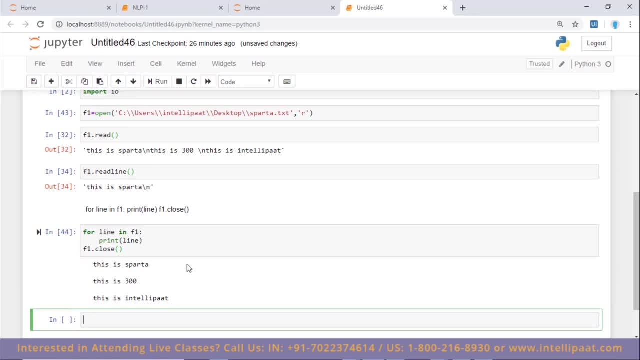 right. so let me run this right, so let me run this right. so i've extracted each of these right, so i've extracted each of these right, so i've extracted each of these lines with the help of the for loop, so lines with the help of the for loop, so 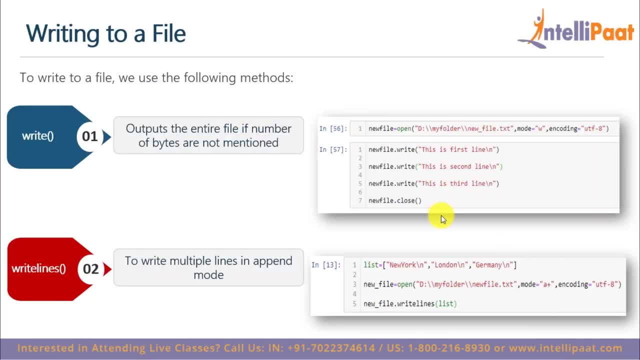 lines with the help of the for loop. so we've got: this is pada, this is 300. and we've got, this is pada, this is 300. and we've got, this is pada, this is 300. and this is intellipath. now let's see how. 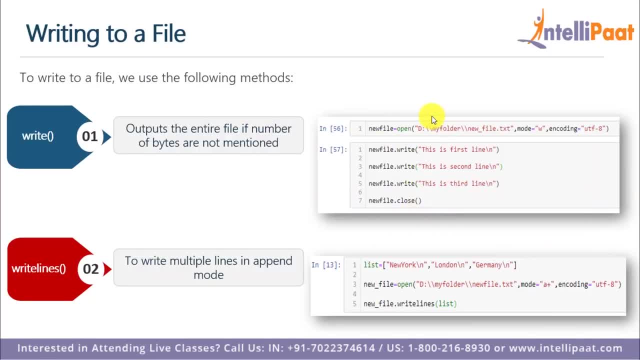 this is intellipath. now let's see how this is intellipath. now let's see how can we write something to a file. can we write something to a file? can we write something to a file? so, to write something to a file we can. 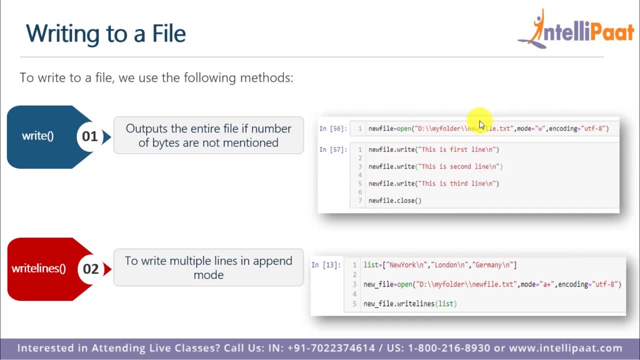 so to write something to a file, we can. so to write something to a file, we can use the right method. so again, we'd have use the right method. so again we'd have use the right method. so again, we'd have to start off by opening the file. but 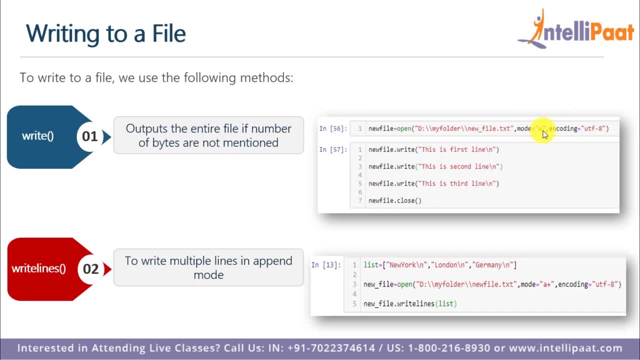 to start off by opening the file. but to start off by opening the file, but this time we'll be opening this. in this time we'll be opening this in this time we'll be opening this in right mode. so over here i'll set mode is right mode. so over here i'll set mode is. 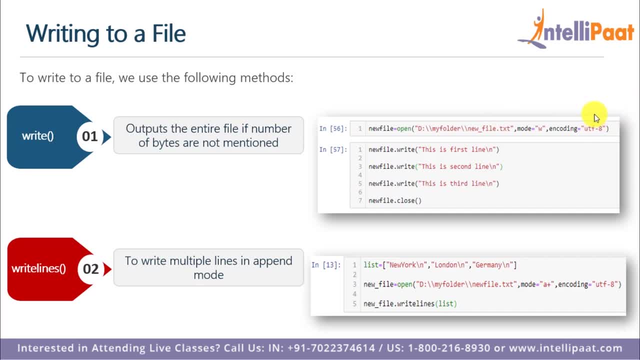 right mode. so over here i'll set: mode is equal to w, equal to w, equal to w, and. while writing, i also have to set the. and. while writing, i also have to set the. and. while writing, i also have to set the encoding type. so the encoding of this. 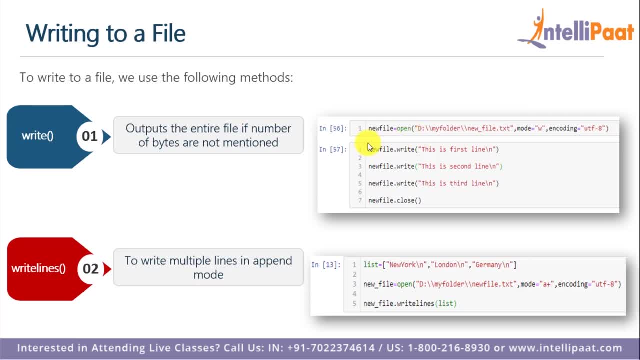 encoding type. so the encoding of this encoding type. so the encoding of this file is utf-8, and what i'll do is i'll file is utf-8 and what i'll do is i'll file is utf-8 and what i'll do is i'll add three new lines over here, so i'll. add three new lines over here. so i'll add three new lines over here. so i'll type in: this is the first line. this is type in. this is the first line. this is type in. this is the first line, this is the second line and this is the third. 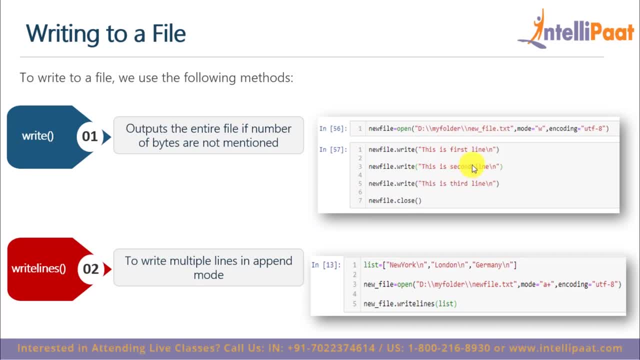 the second line and this is the third, the second line and this is the third line, and these three would be added to line and these three would be added to line, and these three would be added to this current file now, instead of adding this current file now, instead of adding. 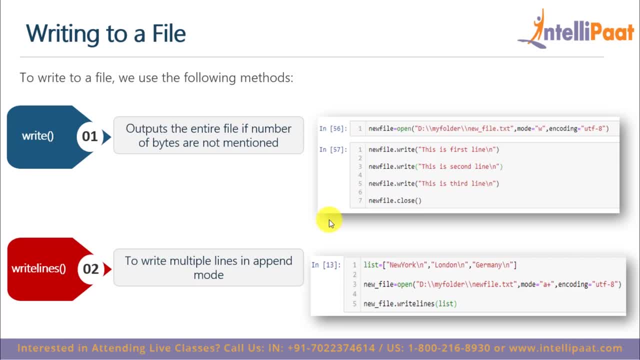 this current file. now, instead of adding one single line, let's say, if i wanted to one single line. let's say, if i wanted to one single line. let's say, if i wanted to add multiple lines over here, so for this. add multiple lines over here, so for this. 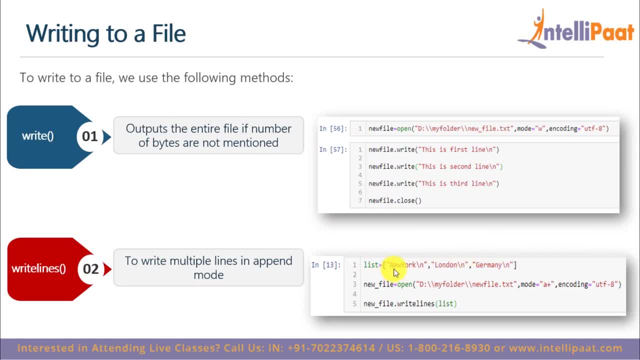 add multiple lines over here. so for this, what i'd have to do is i'll create a. what i'd have to do is i'll create a. what i'd have to do is i'll create a list and inside this list, i'll separate list and inside this list, i'll separate. 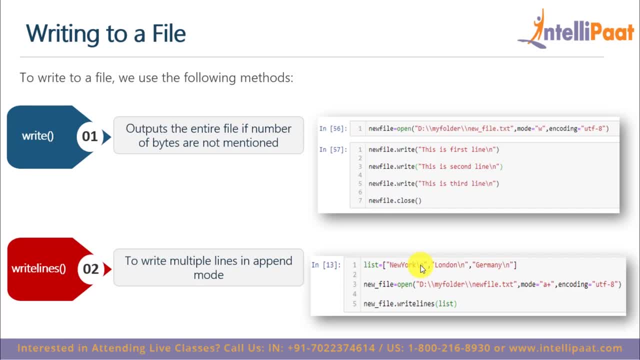 list and, inside this list, i'll separate these three items. with the help of these three items, with the help of these three items, with the help of slash in so as we already know, this slash in so as we already know, this slash in so as we already know, this slash in it denotes a new line. 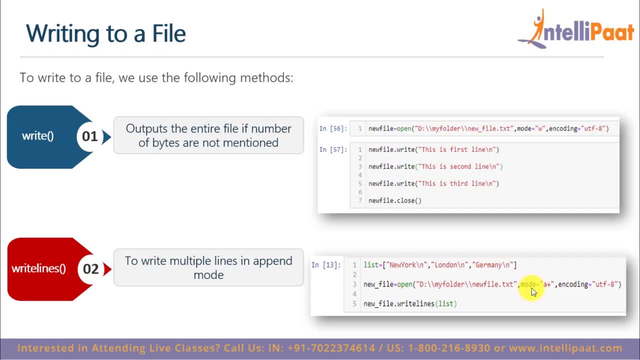 slash in it denotes a new line. slash in it denotes a new line right now. after that, we'll open the file right now. after that, we'll open the file right now. after that, we'll open the file and over here, we'll open this in the. and over here, we'll open this in the. 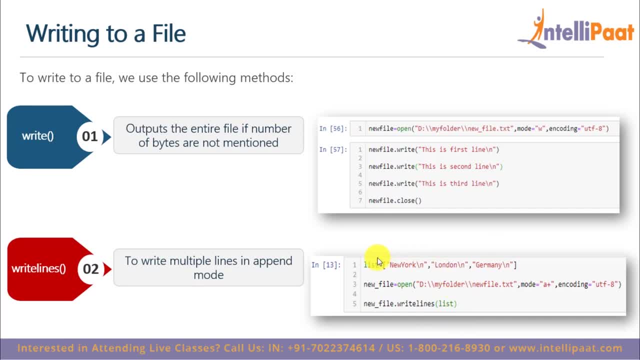 and over here. we'll open this in the mode a plus. so a plus stands for the mode a plus. so a plus stands for the mode a plus. so a plus stands for the append mode, and we'll write this entire append mode and we'll write this entire. 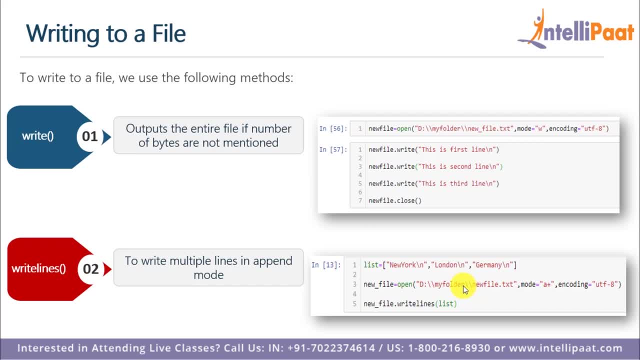 append mode and we'll write this entire list into the file over here now. let's list into the file over here now. let's list into the file over here now. let's perform these operations right. so what perform these operations right? so what perform these operations right? so what i'll do is i'll copy the same command. 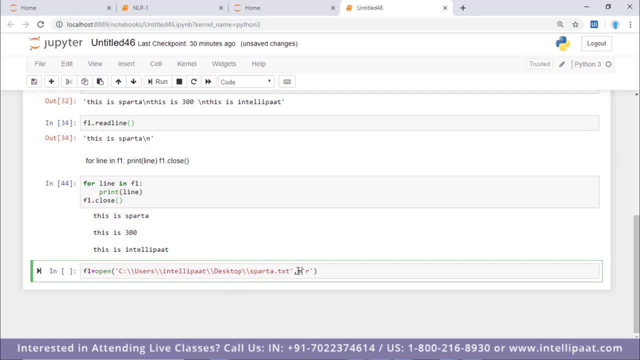 i'll do is i'll copy the same command. i'll do is i'll copy the same command over here and paste it over here. so the over here and paste it over here. so the over here and paste it over here, so the file would be the same. 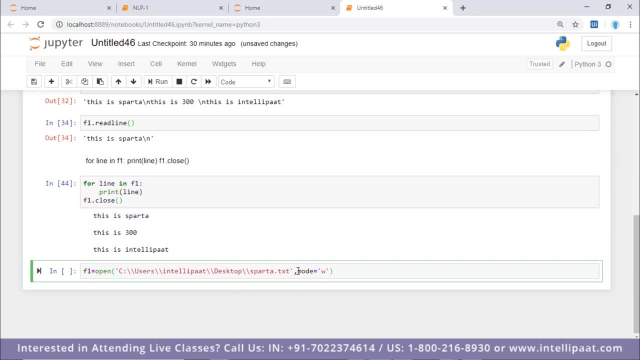 file would be the same. file would be the same, and over here i'll set the mode to be, and over here i'll set the mode to be, and over here i'll set the mode to be: equal to w, so w stands for right, and equal to w, so w stands for right. and. 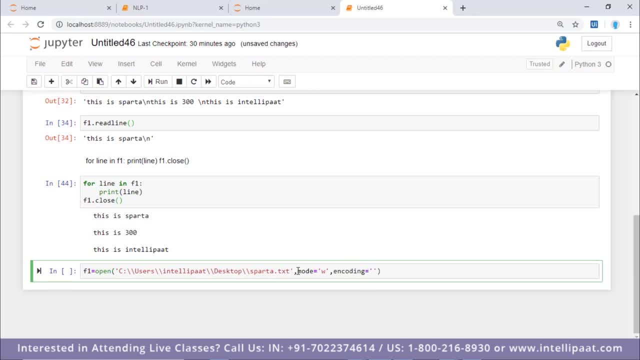 equal to w, so w stands for right. and after this i'd have to set the encoding. after this i'd have to set the encoding, so encoding would be equal to utf-8. so i'll type in utf-8 over here and i'll click on run. 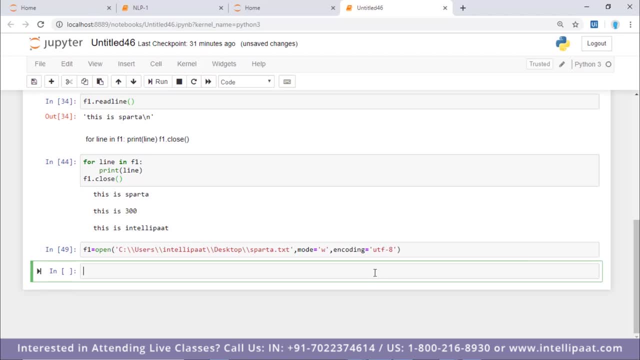 right. so i've successfully opened this file in write mode. now i'd have to go ahead and write something into this. so i'll type in f1 dot right over here and let me write something inside this. so let me add the first line over here. so the first line would be: this is one i'll click on: run. 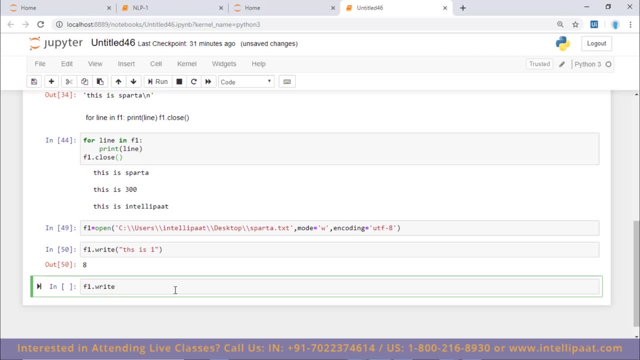 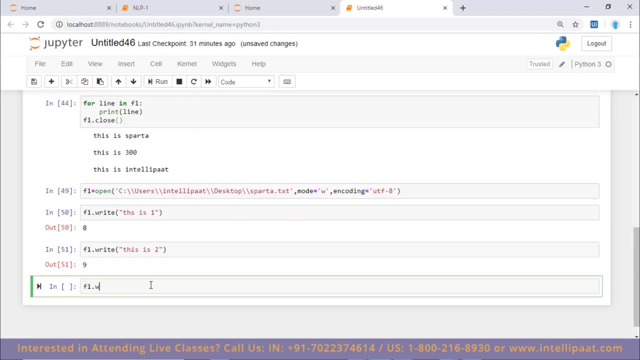 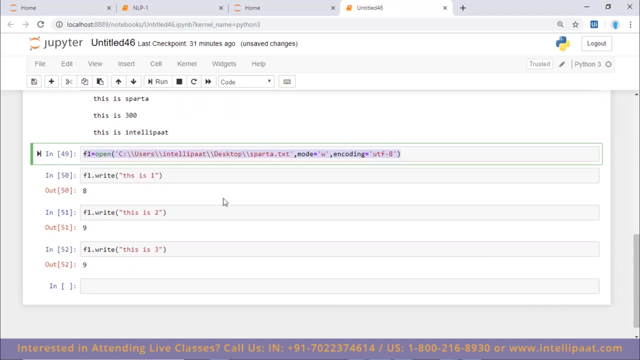 then i'll type: let's say f1, dot. right, and i'll type: this is two. i'll click on run again, then i'll type f1, dot right, and i'll add the line: this is three. now let me go ahead and open the file. so this time i'll open the file in read only mode. so i'll set this mode to be equal to r and 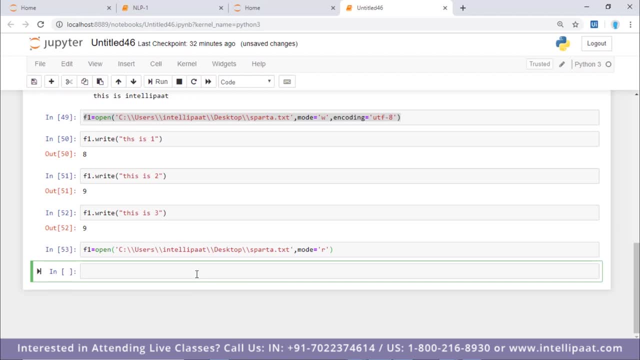 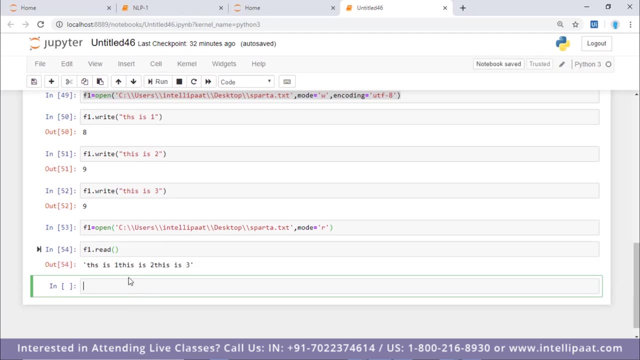 i'll remove the encoding from over here. i'll click on run. right now i'd have to type in f1 dot read, right. so this is what i have. this is one, this is two and this is three. right, so i've successfully added these three elements into my file. now, as you see, over, 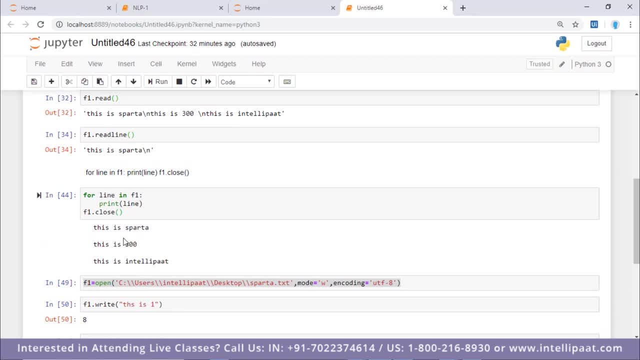 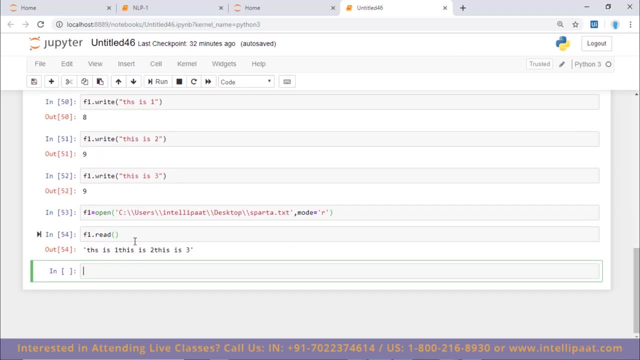 here. my file initially had these three lines over here. this is part of, this is 300 and this is in telepath. now, when we use the write mode and we entered these three lines- this is one, this is two and this is three- what it did was it replaced these three lines with this and this. 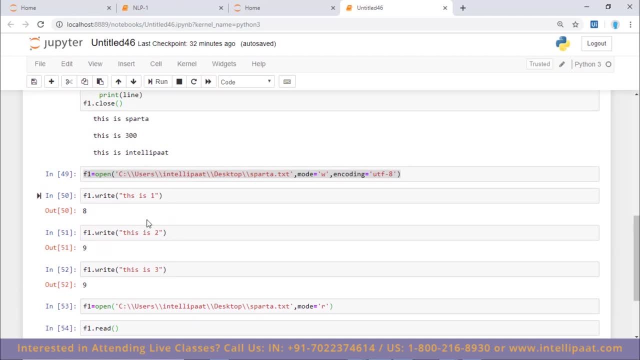 has a little bit of a difference between the two lines. so this is one, this is two and this is three. this is one, this is b. right, these are the two lines that the pointer had formed and for that whole process. and this happen because the pointer starts at the beginning of the file and when the 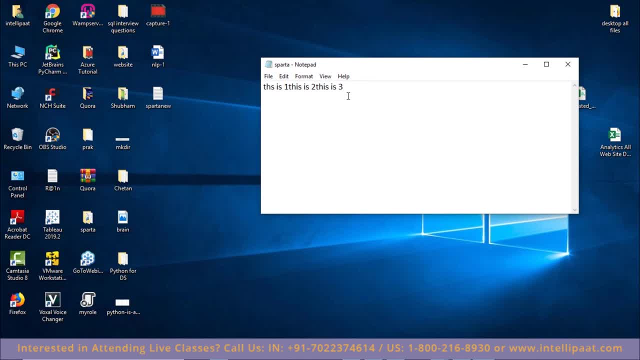 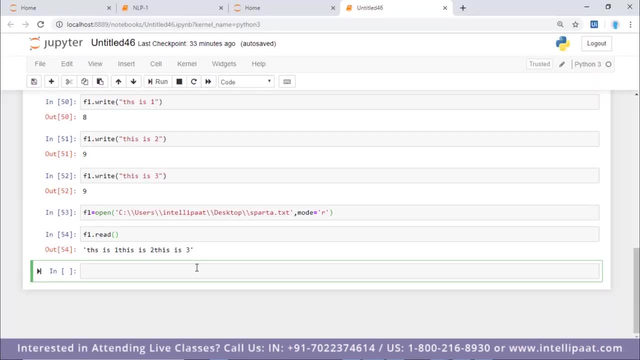 pointer starts at the beginning of the file. all that which was there initially, that would be replaced. so l if i go to the file now and see how it looks like, right? so i have a single line now. this is one, this is two and this is three, because the earlier thing was replaced. now i'll go ahead. 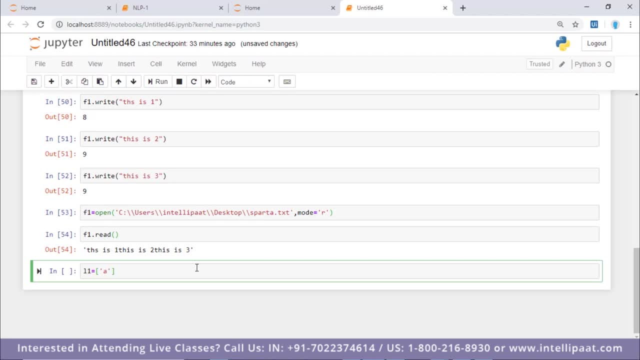 and actually create a list over here. so i'll name this as l1 and i'll add some values over here. so line after this. then the second value is b. again i'll add a new line after this and then i'll add a new value which is c. after that i'll add a new line. now i'll. 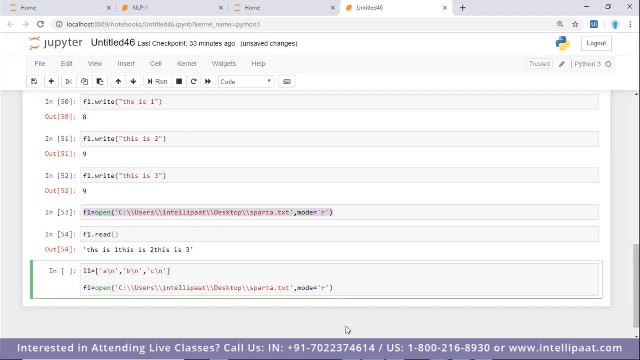 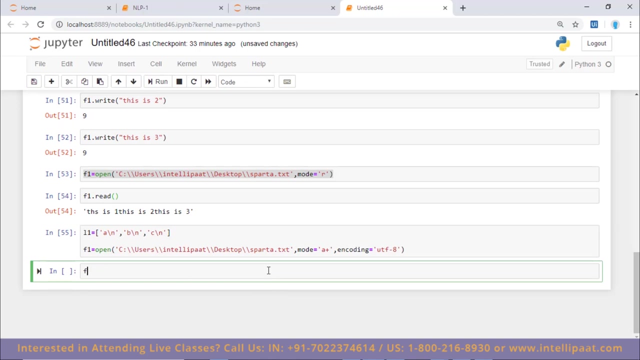 open this file in append mode. so this would be the same. the mode would be a plus and i'd have to give the encoding again. so encoding would be utf-8, right. so this time i've opened the file in append mode. now what i'll do is i will go ahead and add this, so 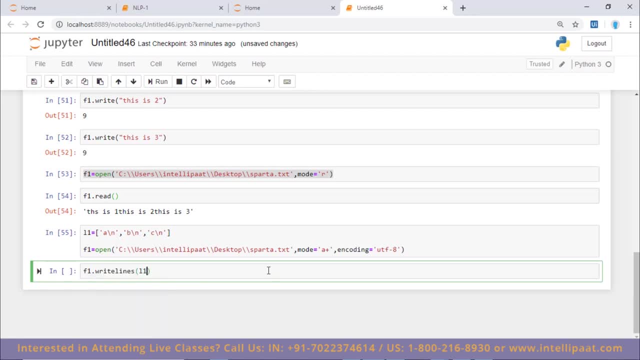 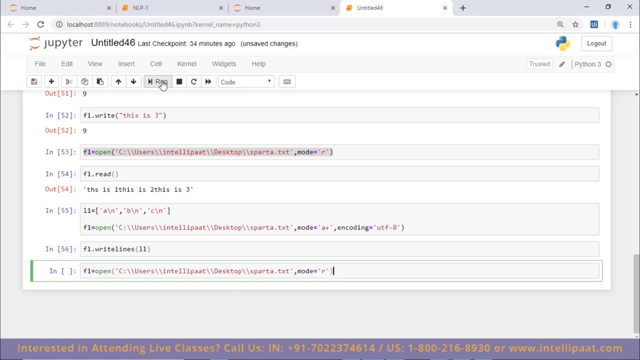 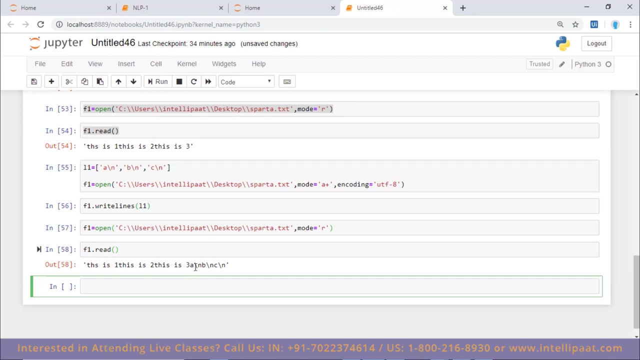 write lines and inside this i'll just put in l1. now i'll go ahead and open the file. let's see what do we get. so i'm opening the file in read mode now. now let me read what we have in this file. so now i have successfully added. 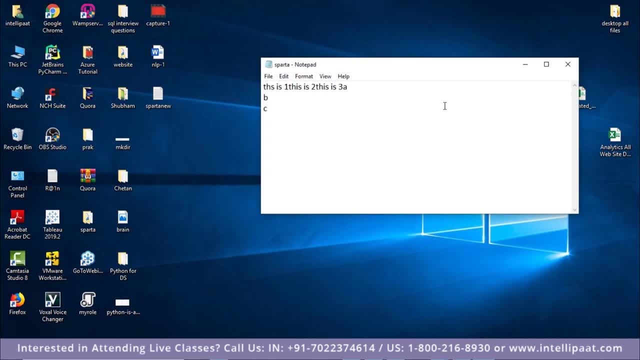 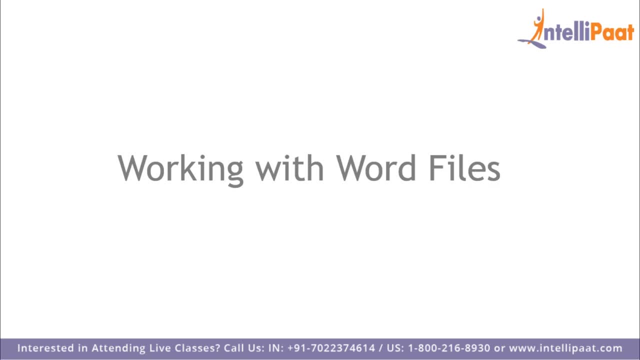 these three characters over here: a, b and c. so now let me open the file, right? so this was the first line. after that i added a, b and c. all right, guys. now let's see how can we work with word document file. so we have this library with the name python docx and we can use this for. 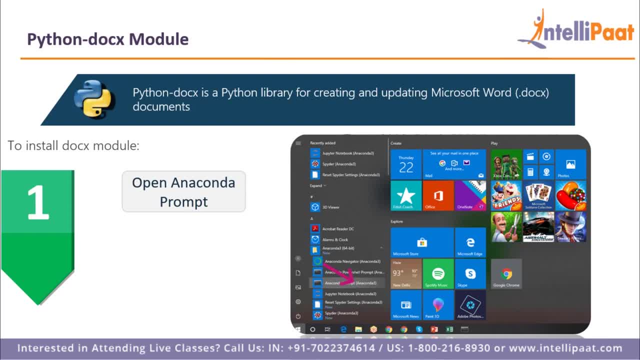 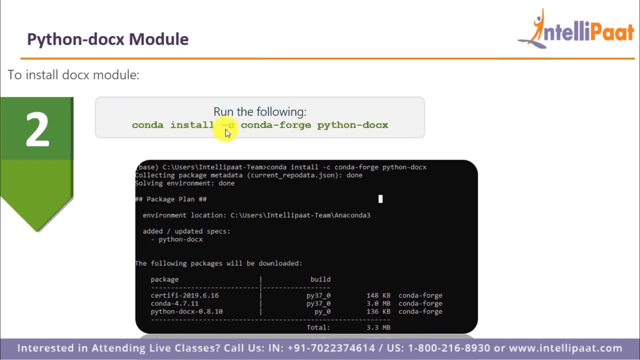 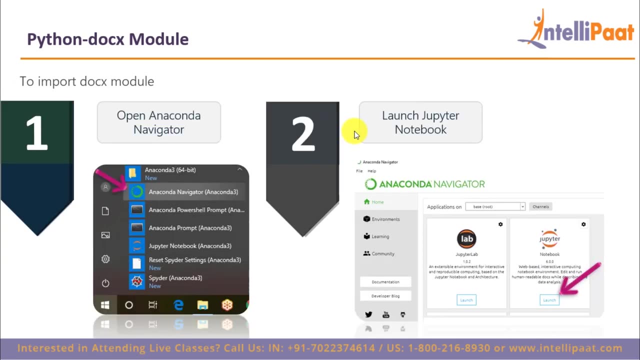 creating and updating microsoft word documents. so to install this library we again have to go to anaconda prompt, and inside anaconda prompt we'll given this command: conda install hyphen c. conda forge python docx- right. so with the help of this command we'll be installing python docx library. so once the 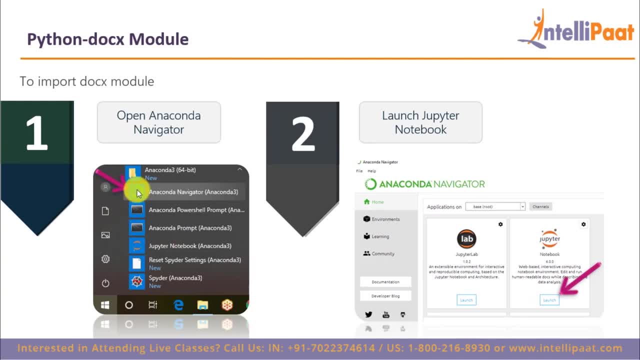 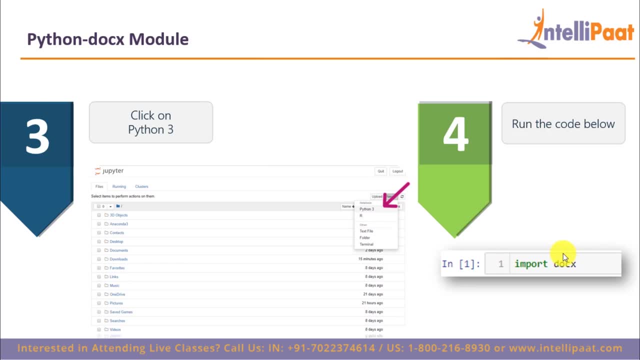 installation is done, we'll go to either anaconda prompt or anaconda navigator and then launch the jupyter notebook. so we'll open a new notebook over here, new python notebook, and we'll type in: import docx. so here you have to keep in mind that when importing the library you'd have to type docx and not 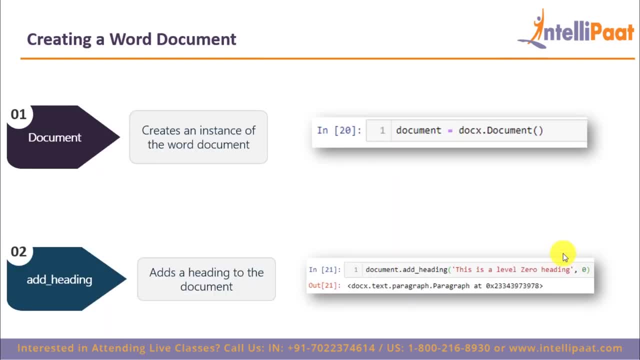 python, docx. so you'll type in import, docx. so once you import the library, now let's see how can we create and update a word document. so, starting off, we'd have to create an instance of our word document. so to create an instance, we'll invoke the document method. so we'll type in: docx, dot. 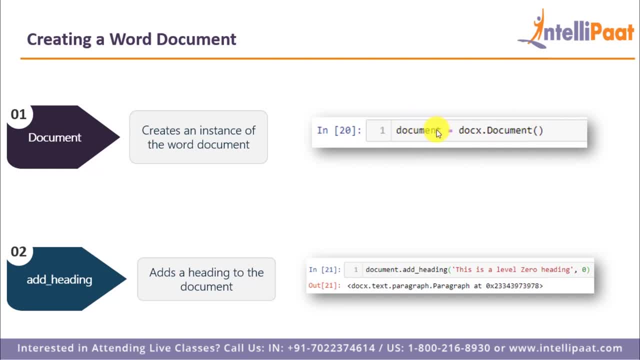 document and we'll create an instance of the word document, so i'm naming this instance as document. now, once we have this instance, we can add all of the content into our word document. so i'll type in document dot- add heading and with the help of this, i can add a heading to. 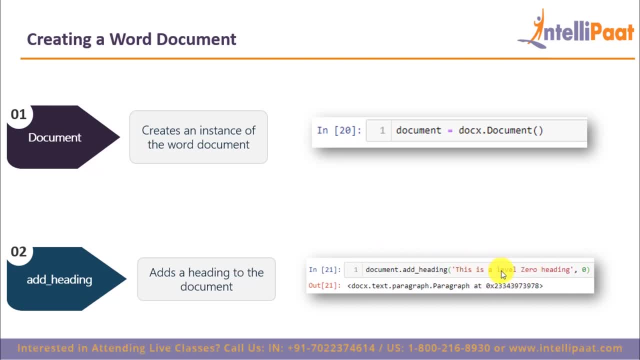 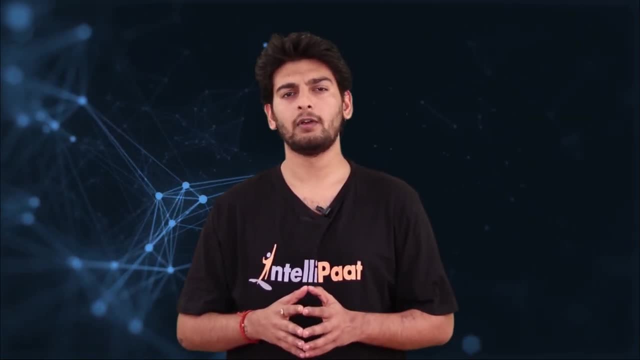 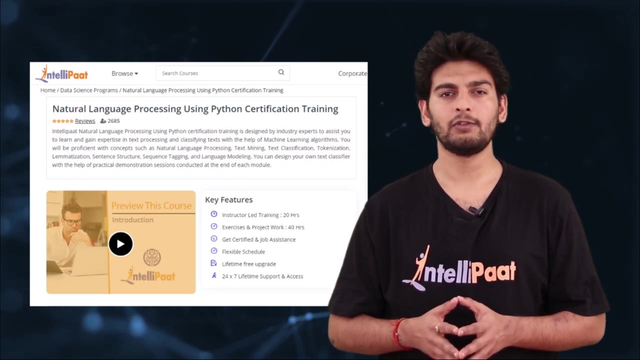 my document right, so over here i'm adding the heading. this is a zero level heading, so here zero indicates the level of the heading. right, right guys? so just a quick info. if you're interested in doing an end-to-end certification in nlp, then intel bar provides the natural language processing training course so you can check out the course. 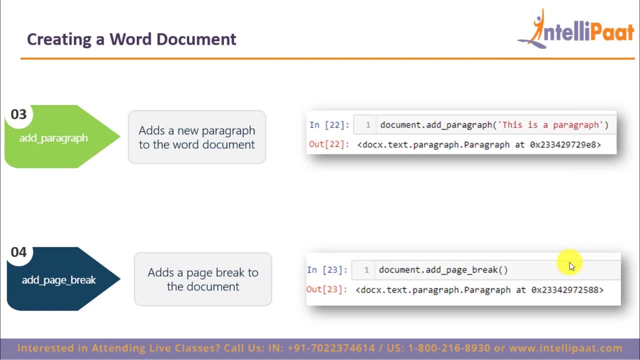 details in the description below. so let's continue with the class. so once we add the heading, now we are going ahead and adding a new paragraph. so here i'm typing document dot, add paragraph and i'm just writing: this is a paragraph and after that, if i want to add a page break so we can use. 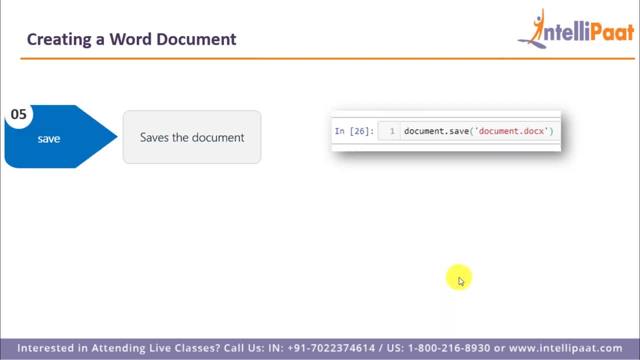 this method: document dot add- page break. so we created an instance and with the help of that instance we added a heading and we also added a paragraph. now it's time to save the document. so to save the document, we'll type in document dot add. paragraph dot save, and inside this we'll give in the name by which we want to save the document. so i'm 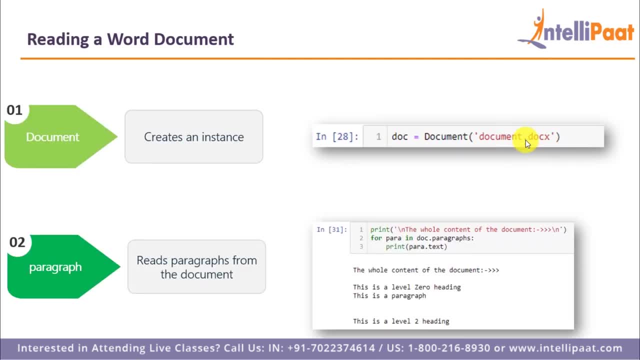 saying the document as document: dot, docx. right, so this is how we can create a document. now let's see how can we read a word document. so to read a document, we'd have to start off by importing this document method from docx and then we'll use this document method and inside this we'll pass in the 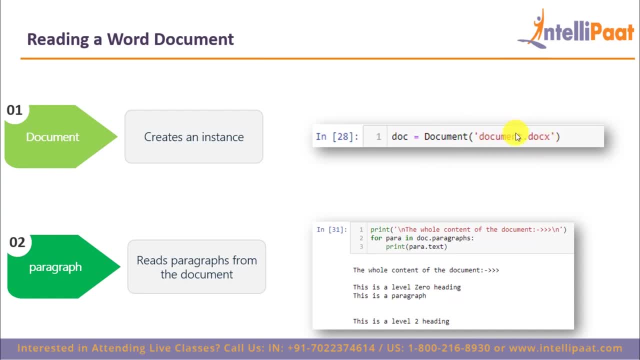 name of the document. so we'll pass in document dot, docx and this is the file which i had just created earlier, and we'll save this in a new instance and name that to be doc. so once we have this instance over here, we'll use the for loop and with the help of this for loop we'll print all of. 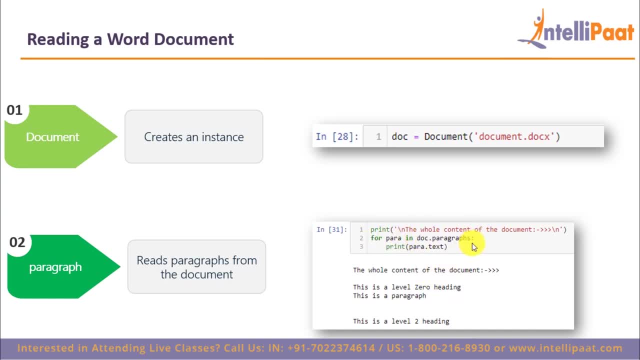 the content inside this document. so i'm typing in for para and doc dot paragraphs: print para dot text. right, so we'll take in each paragraph over here and it will print each paragraph with the help of this for loop. right now let's go to jupyter notebook and actually perform this. so i'll start. 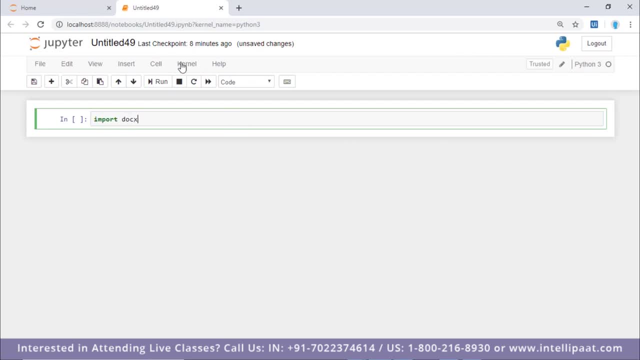 by importing the library, which is docx. so i'll type in import, docx. now i'll go ahead and create an instance of this, so docx, dot, document, and i'll name the instance as doc. so now that i have the instance, i can add the content into this. 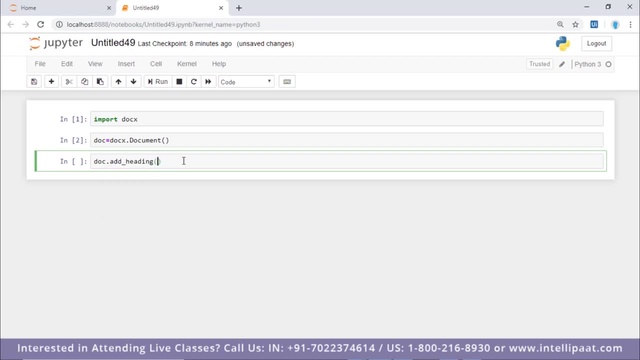 so i'll type in doc- dot, add heading. now let me add the heading. so i'll just say heading one over here, and then i'll add a couple of paragraphs. so this time, doc- dot, add paragraph, and inside this i'll type in p1 and then i'll add another paragraph. so i'll type in doc- dot. add paragraph again and i'll add p2 inside this. after this i'll add a page break. so i'll type in doc dot. add page break and i'll click on run. now, after the page break, i'll give another heading. so doc dot. add heading and I'll give the heading as heading 2. 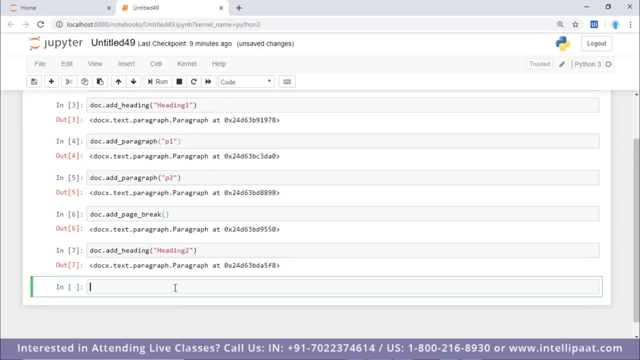 so all of this is done. now it's time to save this document. so I'd have to type in doc, dot, save and I'll give the name of the file. so I will save this as, let's say, my doc dot, doc X, right. so now I have successfully 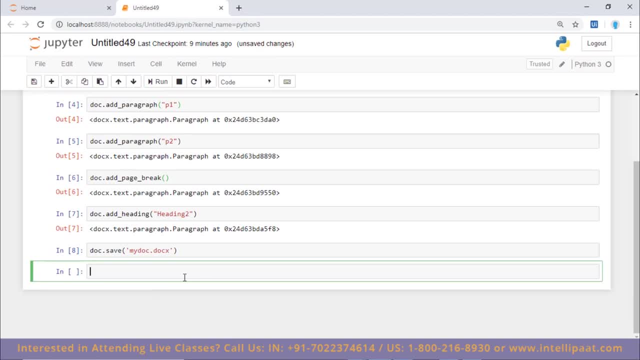 saved this file. now it's time to read this document which have just created. so I'd have to import document. so I'll type in: from doc X, I'd have to import document, right so now that I've imported this, so I'll just given the name of the doc which I've just created. so my doc dot. 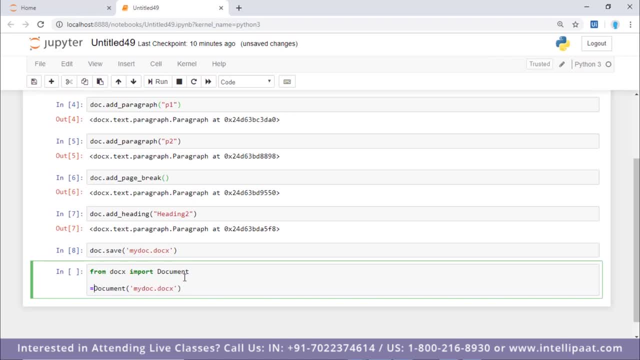 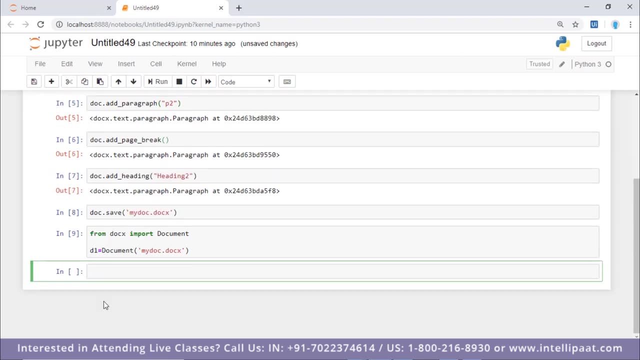 doc X and I'll just will store this in a new document again and I will name this as d1 right. so now I have created a new instance of the document which I had created earlier. now I'll use the for loop, so for para in d1 dot paragraphs. 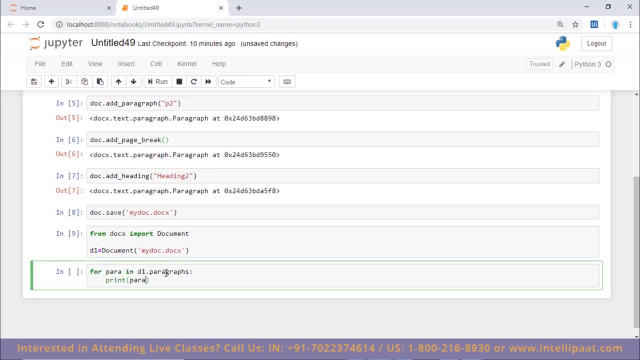 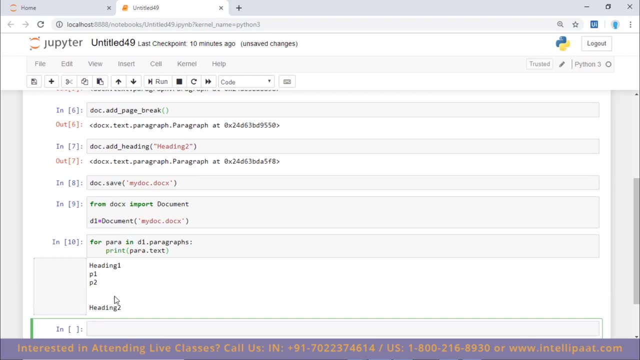 and I'll just print this out. so print a para dot text. so now we have the content which is present in the document over here, heading 1, para 1, para 2, and then we added a page break. after that we have the heading 2, right. so this is how we. 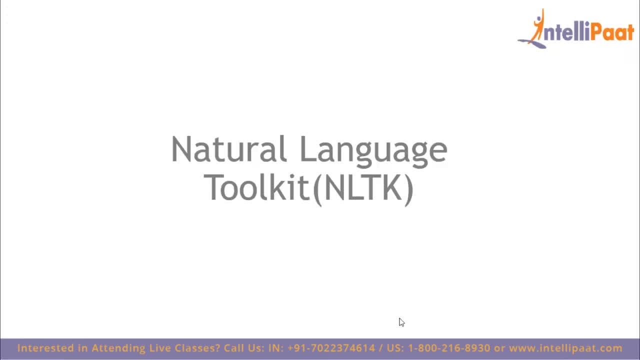 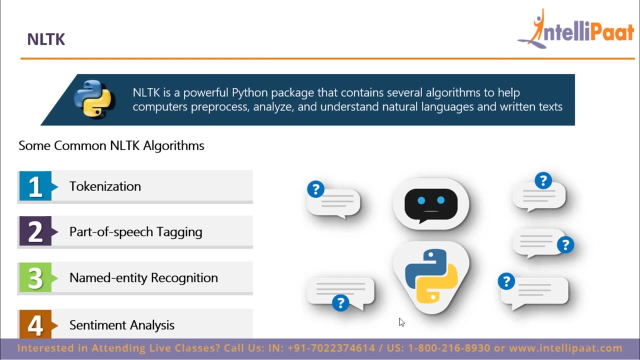 can work with the doc X module. now let's head on to the natural language toolkit. so so NLTK is one of the most widely used packages for the purpose of natural language processing. so NLTK provides multiple packages to perform different operations, such as tokenization, POS tagging, named entity recognition and 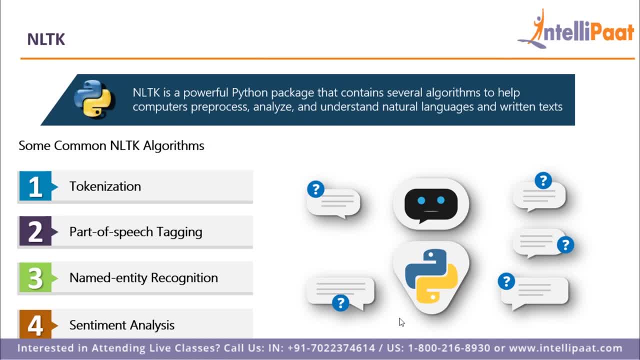 sentiment analysis. right so? NLTK provides very easy and easy to use packages to perform different operations, such as tokenization, POS tagging, named entity recognition and sentiment analysis. right so? NLTK provides very easy to work with modules, and with these modules, all of your work becomes much. 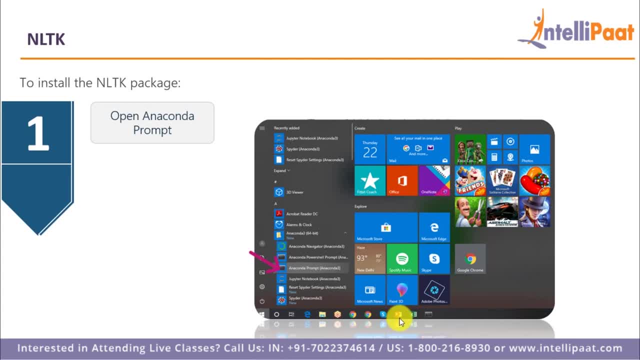 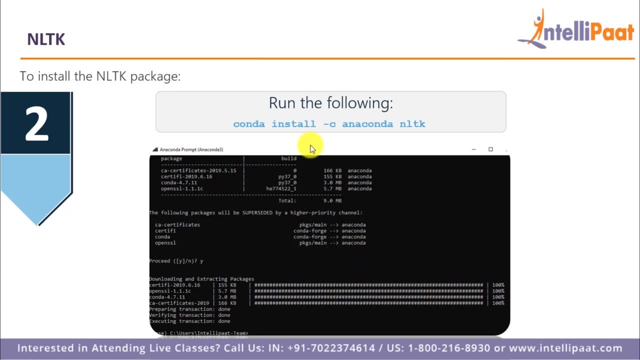 more organized and much more easier. now again, let's see how can we install the NLTK package. so again, we'd have to go to anaconda prompt and we'll give this command inside anaconda prompt over here. so we'd have to type in conda install. 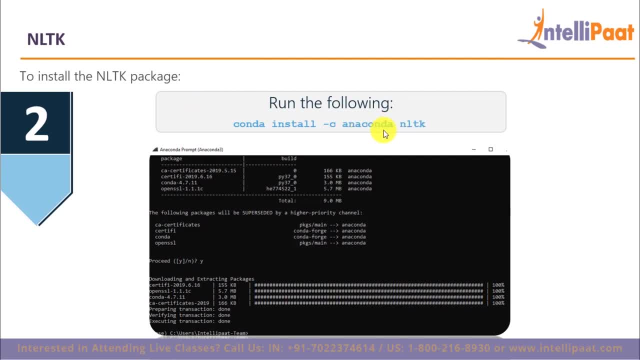 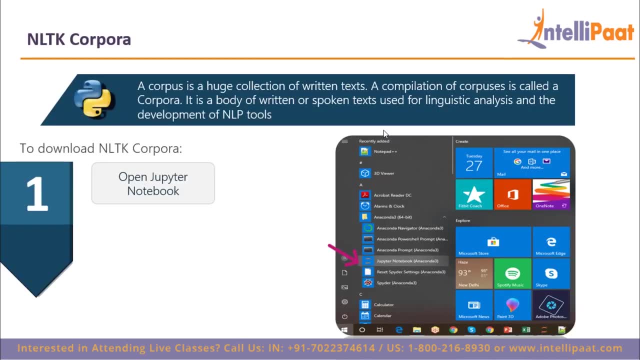 hyphen: see anaconda NLTK. and this is how we can install the NLTK package right now. once we install the NLTK library, we have something known as the NLTK corpora. now you must be wondering: what exactly is a corpora? so before understanding corpora, let's understand what is. 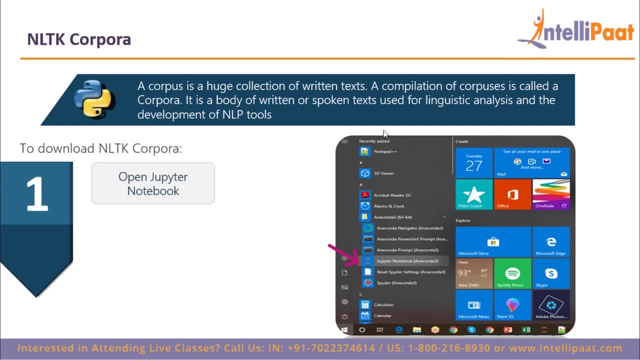 corpus. so a corpus is a huge collection of written text, and the compilation of these corpuses is what is called as a corpora. now, NLTK provides this huge corpora for multiple purposes, so it has got all of these different corpus pertaining to different domains and we can use it to perform various NLP tasks right now. 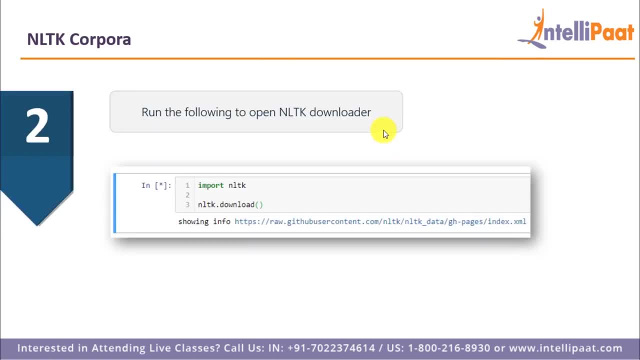 let's see how can we download this NLTK corpora. so once we install NLTK, we have have to go to jupyter notebook and then type in import nltk and then after that we just have to type in nltkdownload. so this would give you a setup wizard. now all you have to do is click on. 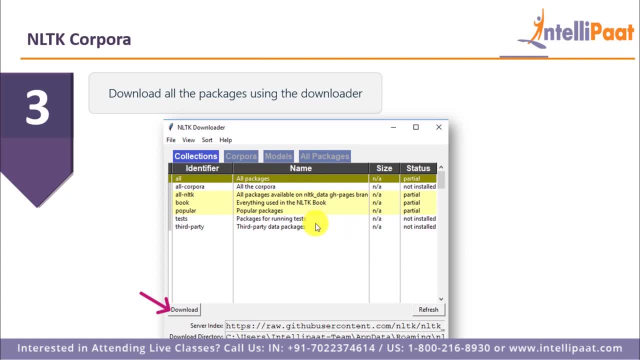 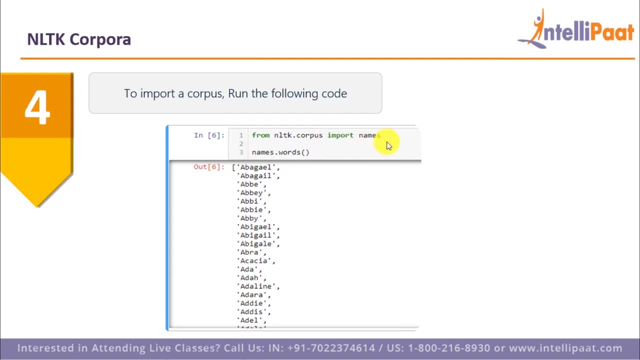 download and this will install all of the corpuses which are present in nltk. so this is how you can import a corpus from nltk. so there's this corpus with the title names and we are importing this corpus. so i'll just type in from nltkcorpus import names, and this just has a list of all. 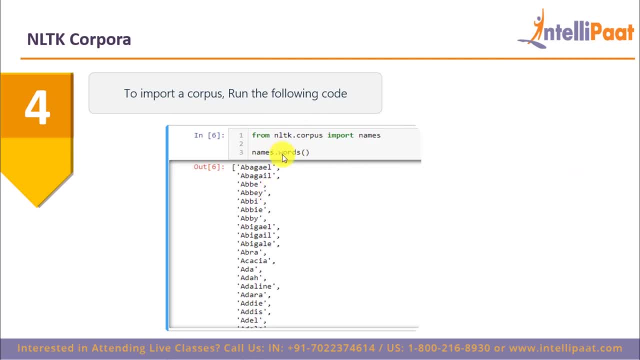 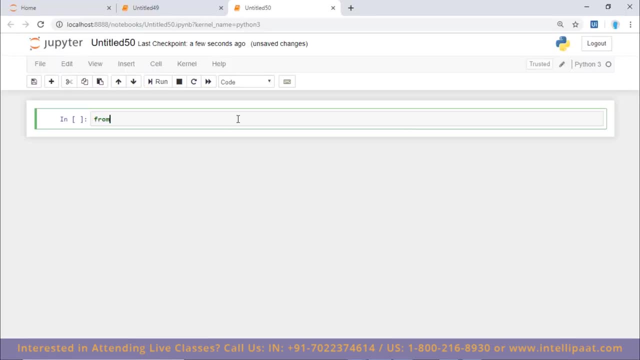 different words. so to have a glance at all of those words, i'll type in nameswords. right now. let me go to jupyter notebook and just show you how can we do this right now. let me start off by importing nltk, so from nltkcorpus. what i want is names, so this is basically the name of the. 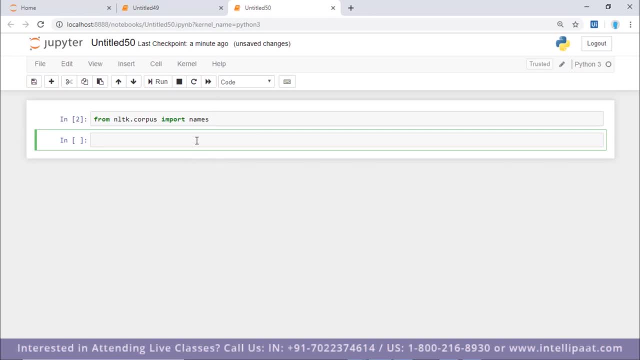 corpus which we are importing right now. i've imported this corpus. now i want to have a glance at the list of the names which are present, so i'll just type in nameswords and i'll click on run. so this is the list of the names which is present inside this corpus. 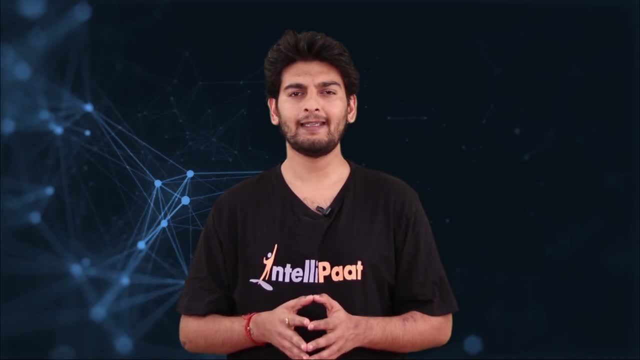 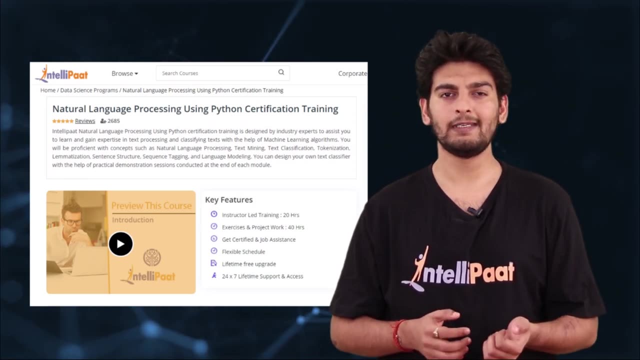 right guys. so just a quick info. if you are interested in doing an end-to-end certification in nlp, then intellipaat provides the natural language processing training course. so you can check out the course details in the description below. right guys? so this brings us to the end of 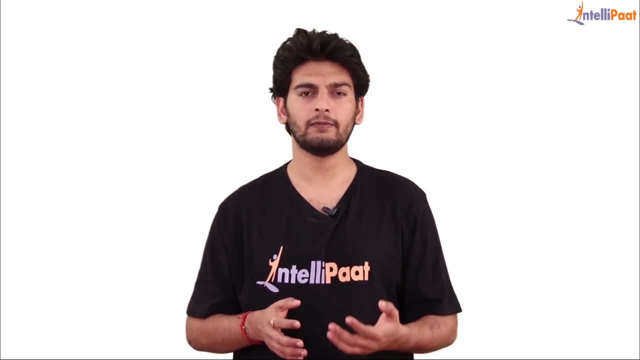 the session on natural language processing. so i hope that you guys have comprehensively learned about natural language processing. also, if you haven't subscribed to our youtube channel, please do it so that you don't miss out on all of our videos. so thank you and happy learning.